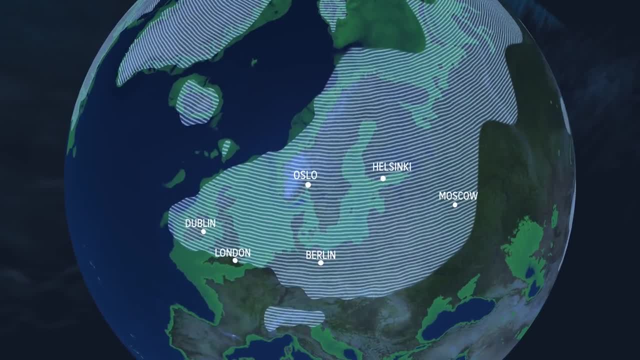 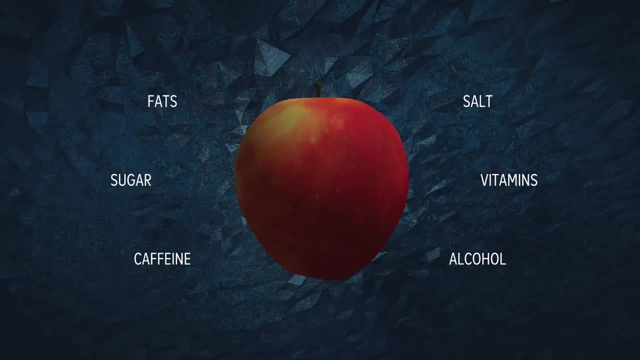 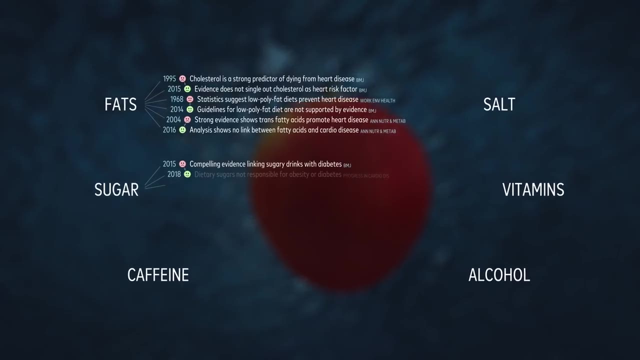 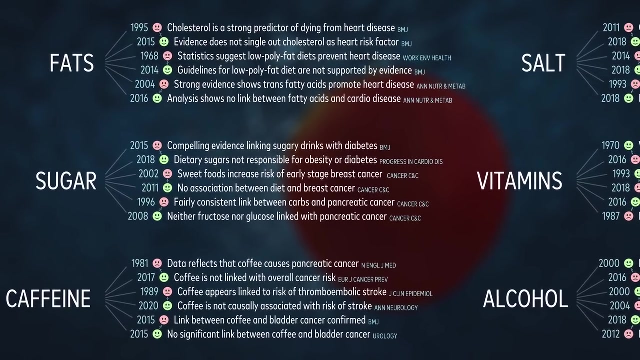 But that's okay, isn't it? To just report what the experts say? Well, Well, the doctor is in on a new study. In some fields of science, like nutrition, the warnings we've received from experts have been unclear By now. we've been told so many conflicting things about which foods will make us live longer, get sick or lose weight that trust has eroded. 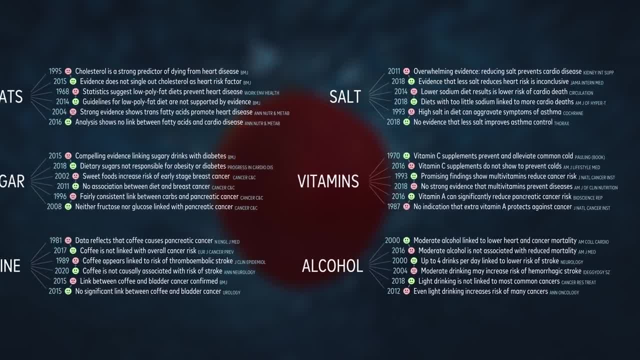 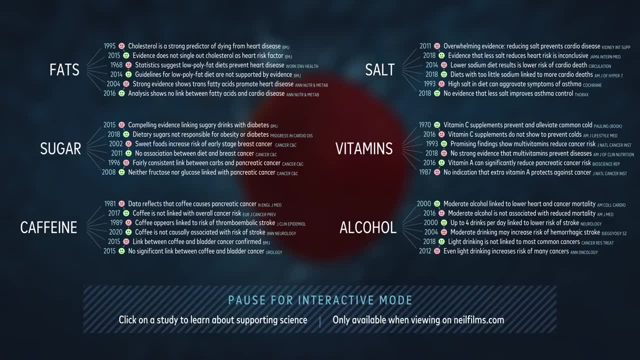 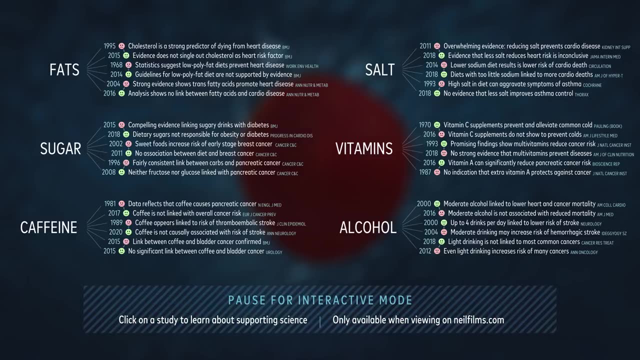 As long as they were fortified with vitamins and minerals. Not anymore. Now we want people to eat the whole food. Now some say junk. Now some journalists are to blame for reporting new health studies without enough explanation about the underlying science. But scientists themselves have apparently been making mistakes, determining how reliable their results are. 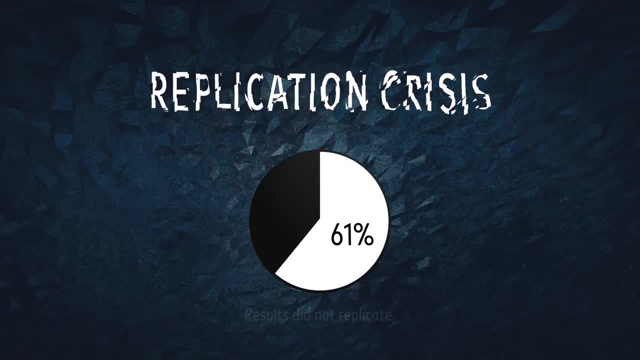 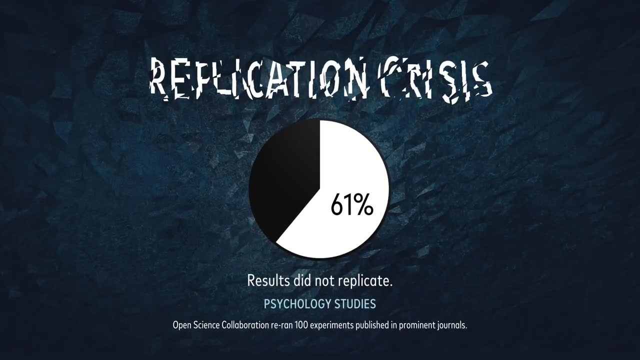 And it's not just newscasters and nutritionists who struggle with uncertainty. We're learning that a significant number of experiments in psychology and some areas of medicine can't be replicated or verified Because the researchers in many cases overstate them. 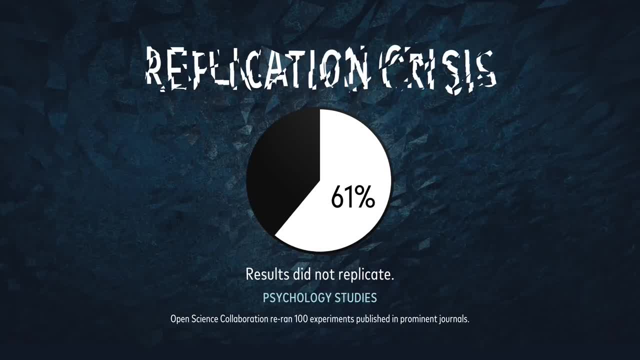 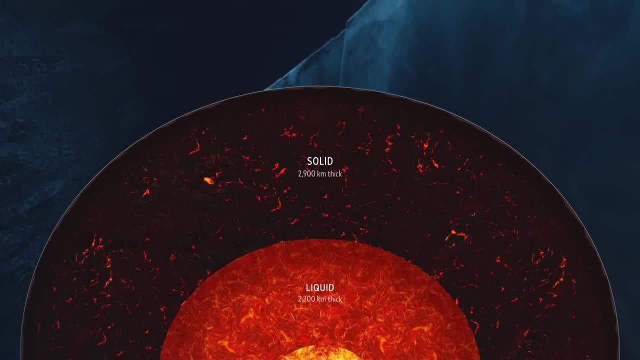 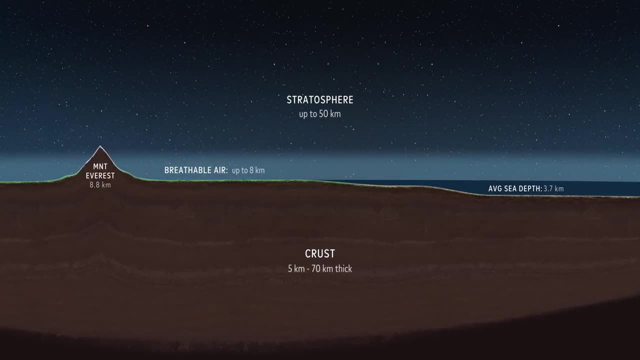 They've just neglected the strength of their findings. Now, on one hand, climate science has a basis in so-called hard sciences like geology and physics, which are less prone to replication problems than research about human behavior, Sometimes called soft science or social science. 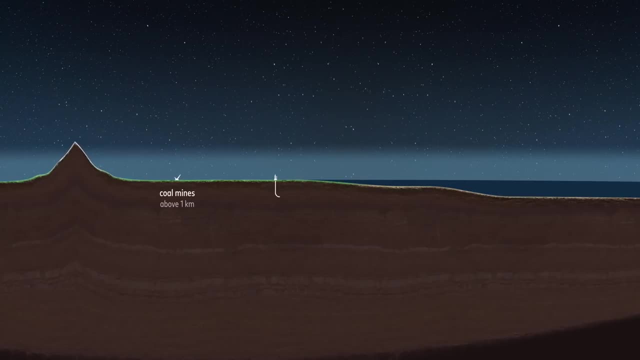 On the other hand, climate change is about humans, right? So do we need both hard and soft science? And how do we make what we harvest out of these hard sciences and soft sciences to understand it? Let's explore this with some carbon arithmetic. 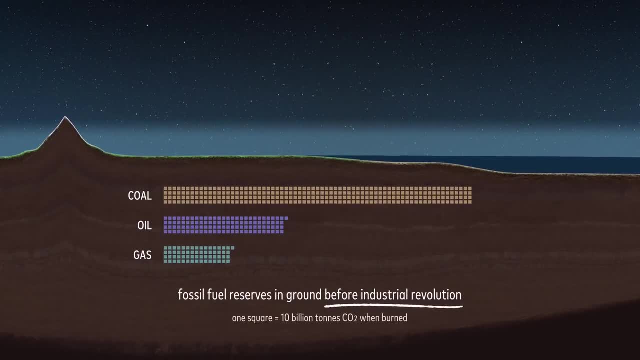 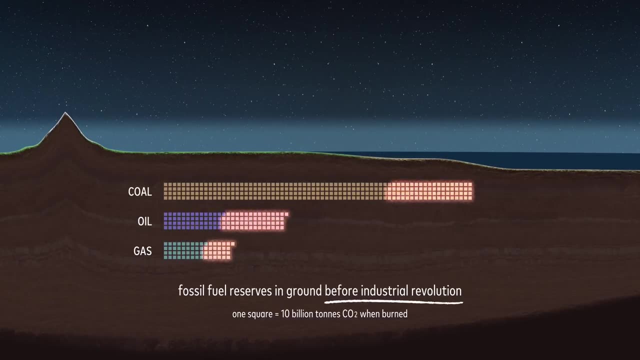 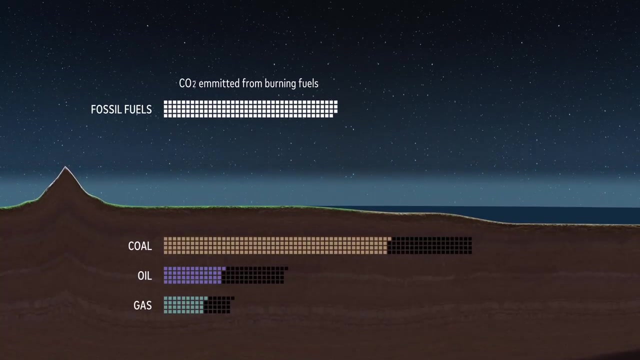 Say we wanted to know how much carbon dioxide has been added to the atmosphere by humans. Well, we know how much fossil fuel has so far been burned And we know how much CO2 would be produced as a result, And we know deforestation releases additional CO2.. 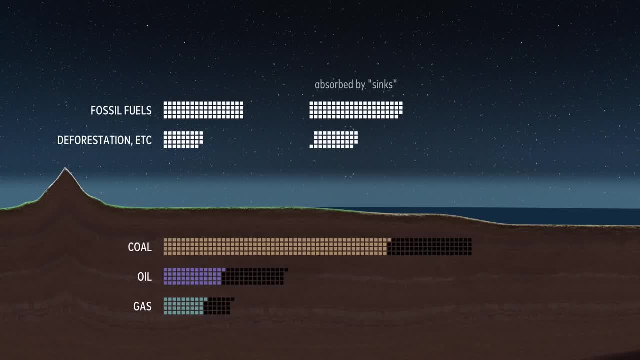 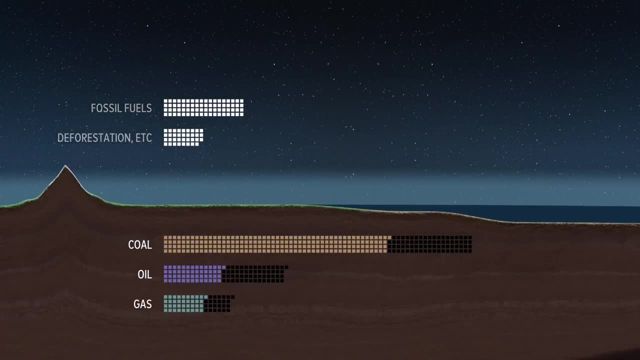 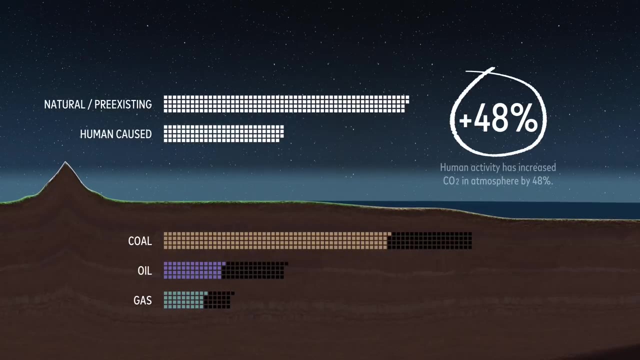 But not all this extra carbon stayed in the atmosphere, because most of it got absorbed by the oceans and soils. Now there is some uncertainty surrounding these numbers, But ultimately we can check our math against air, water and soil samples, grounding our final answer. 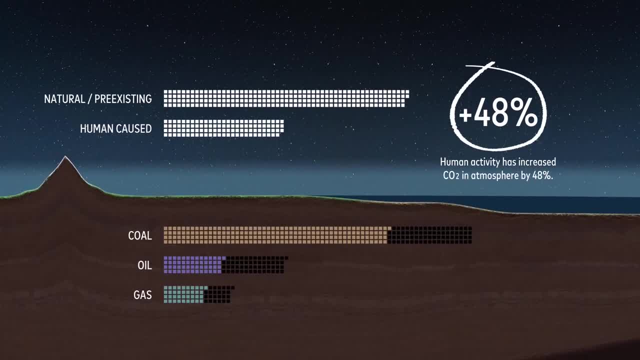 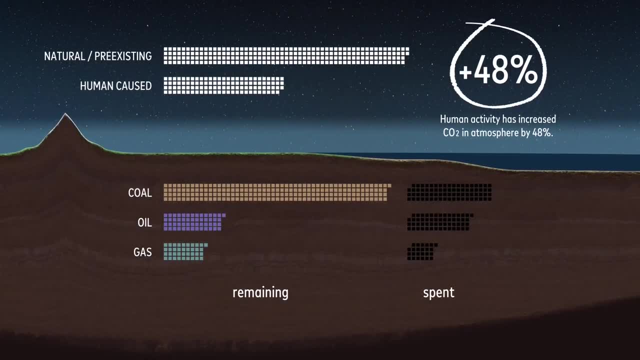 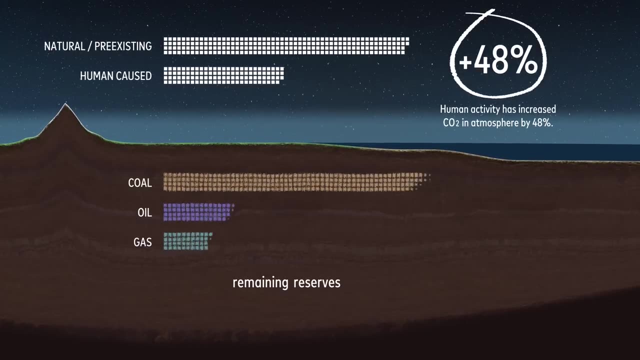 in hard science evidence. But we see the science get softer when we ask a different question: How much fossil fuel is left to economically mine and burn? The Arctic may hold a quarter of the Earth's undiscovered oil. Answering this requires making predictions. 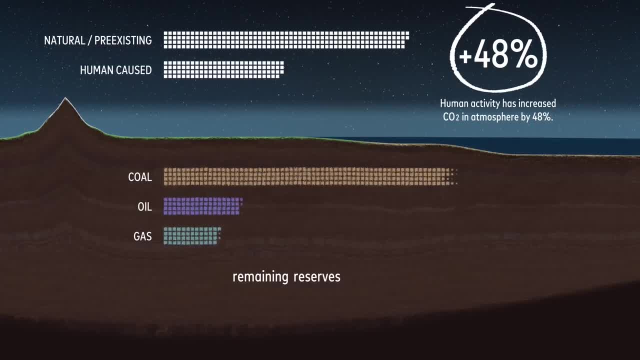 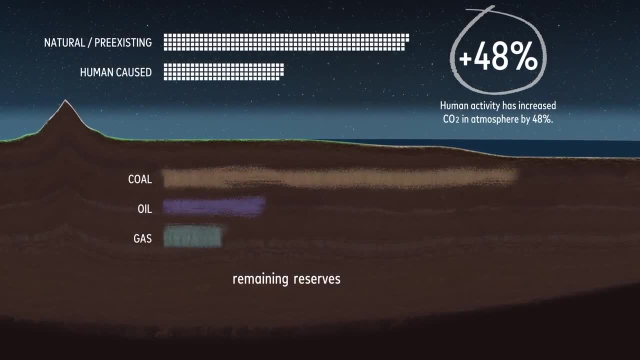 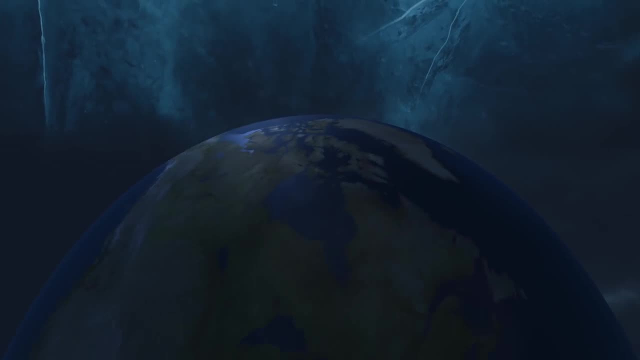 about future discoveries, energy markets and whether countries enact policies that somehow keep fossil fuels in the ground. How much California stands to gain if more fracking is allowed? Categorizing the sciences, like with hard or soft, can be useful if it helps us identify what research is more. 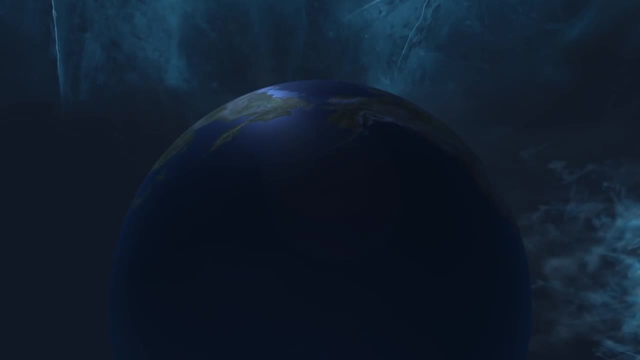 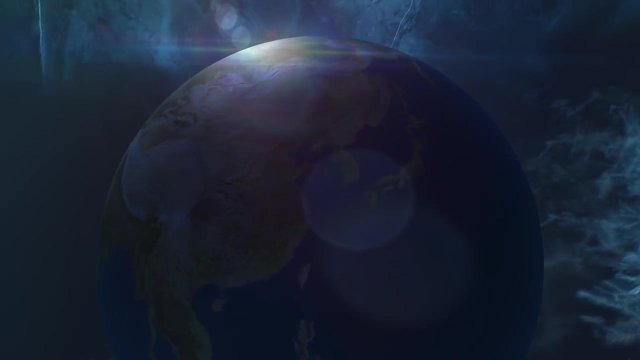 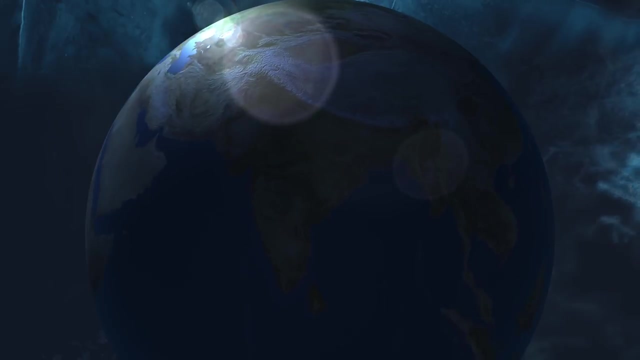 trustworthy, But people studying the replication crisis are still figuring out how widespread it is and what can be done about it. It's a big, active topic of debate, But I'm interested in how journalists and people like me are supposed to report on science. 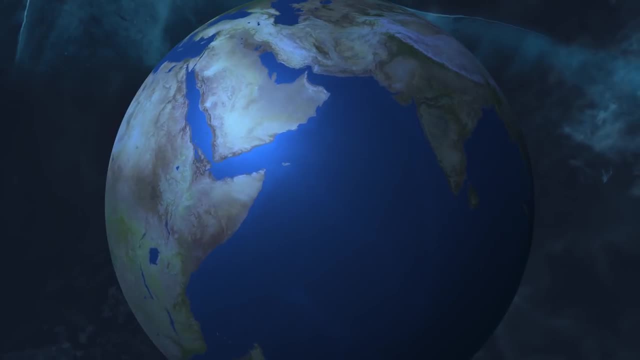 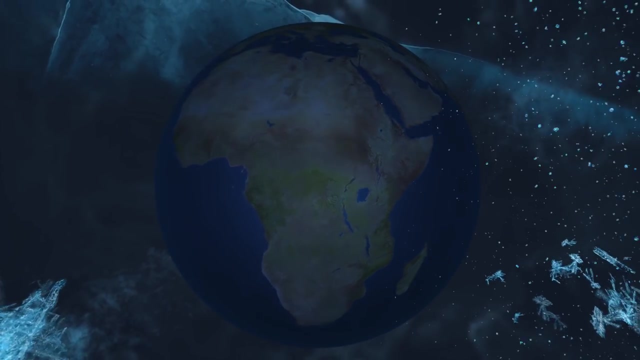 given all these open questions. So here I'll share why I've come to believe that, even when looking at climate research, the only way to learn how sure scientists are is to dig in a little and view their work. with science, I'm going to work with some healthy skepticism. 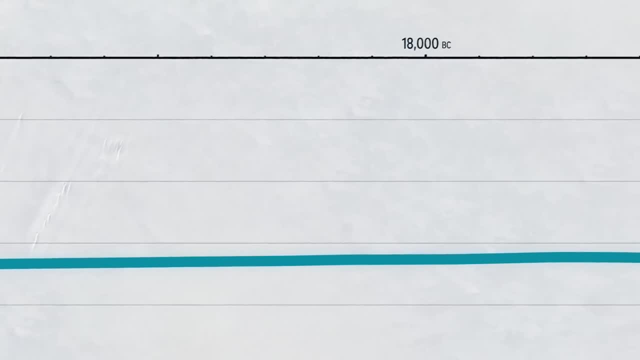 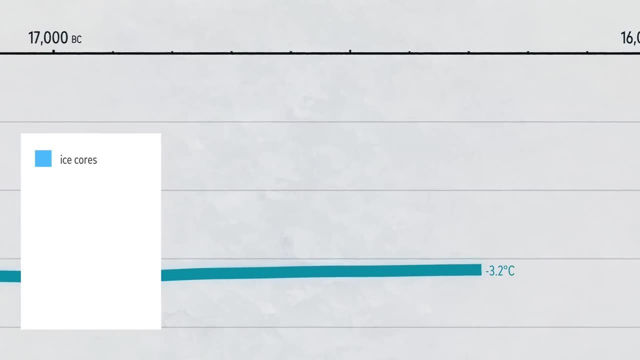 So here we're looking at the Earth's temperature 20,000 years ago. The negative numbers indicate how many degrees colder it was in Celsius than the late 1900s. The temperatures are estimated by looking at ice drilled out of glaciers, as well as fossils such as shells that. 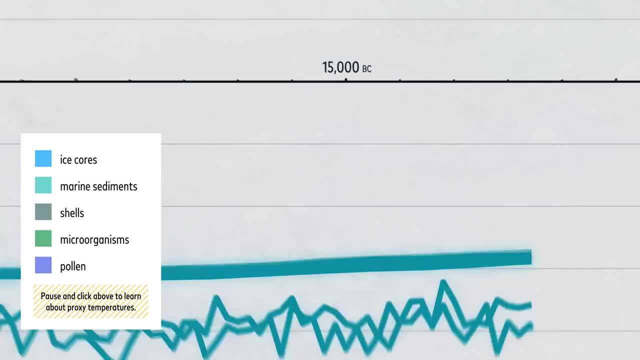 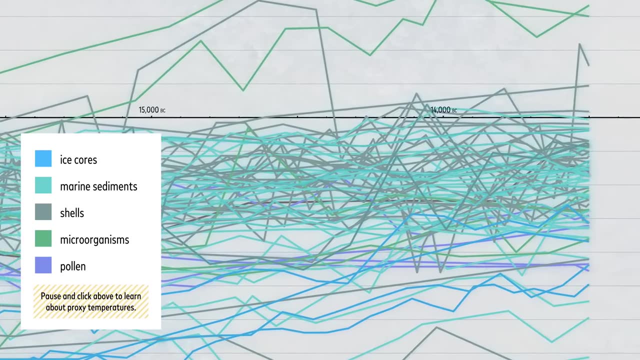 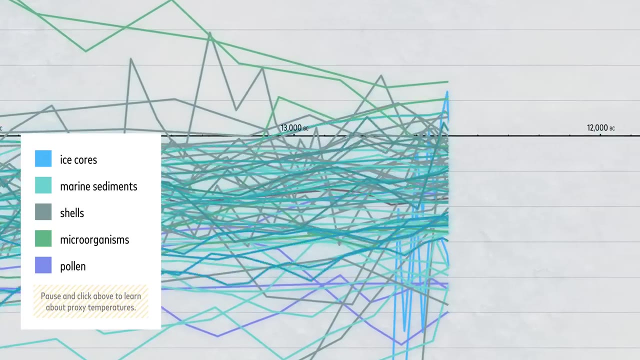 hold clues about the conditions when they are formed, And this particular data comes from a study that combines 80 temperature records from different locations. It's the most comprehensive study I could find for this time period, published in a major journal. The researchers averaged all these messy lines together. 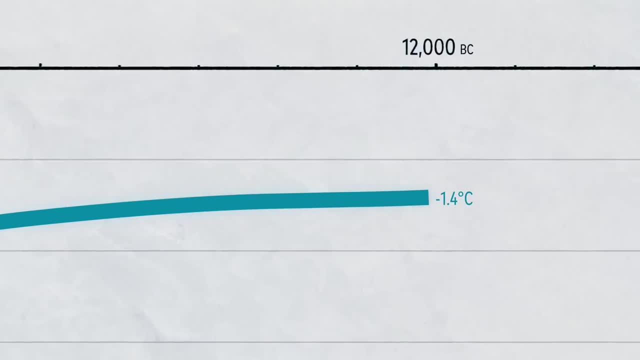 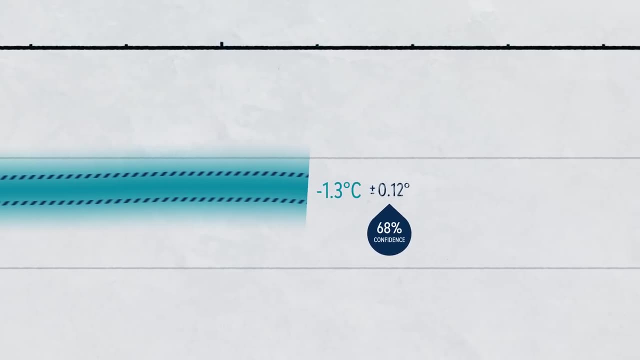 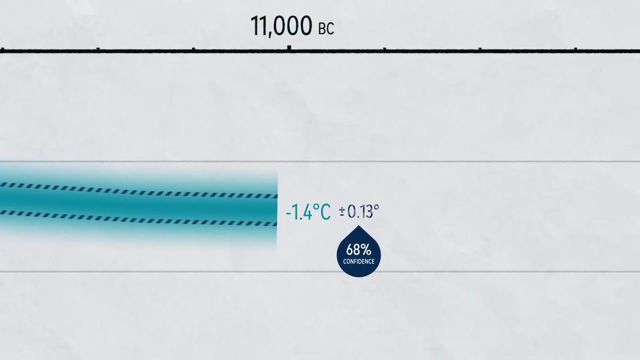 weighing them differently based on location and other factors, And they expressed their confidence level using a margin of error, in this case with 68% confidence. But here's a case where the margin of error doesn't seem to mean that much, Because none of the climatologists I spoke to 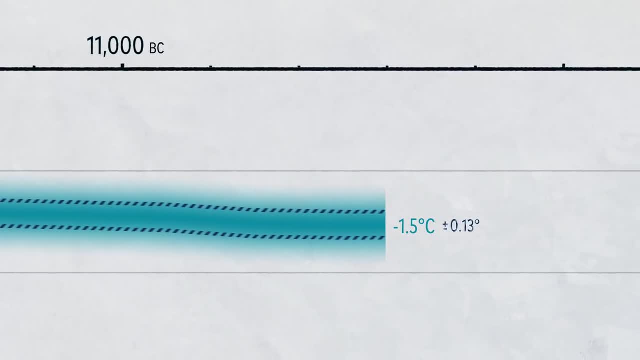 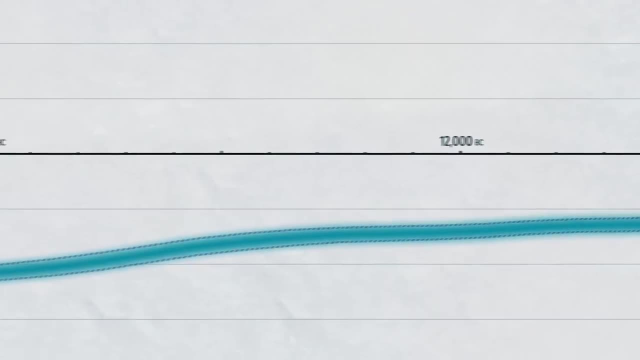 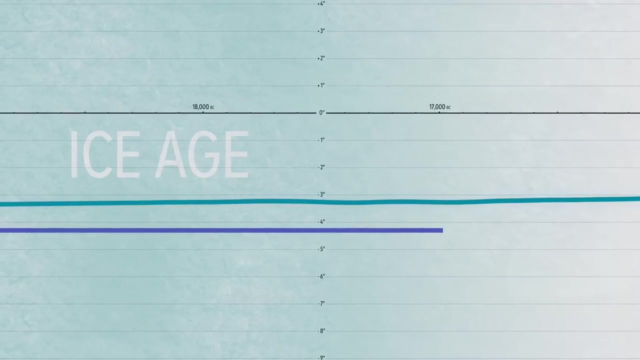 including the authors of this very study, were 68% sure that the true temperature lies between these dashed lines. They all said it's probably lower, Because another study that just focused on the last ice age put the average temperature here. This ice age study is considered to be more reliable. 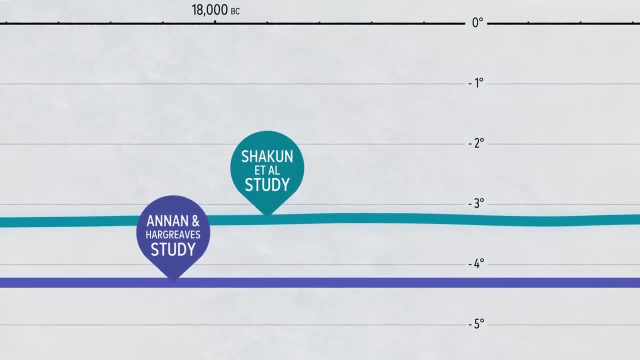 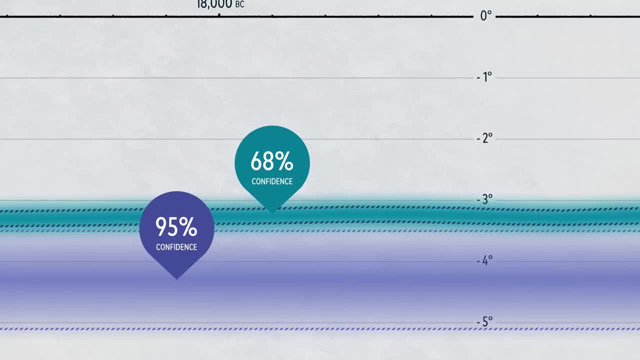 because it factored in more types of evidence and did more robust modeling. Margins of error can be skewed for all sorts of reasons, Which is why talking to scientists can help reveal how sure they really are, And in this case, the climatologists. 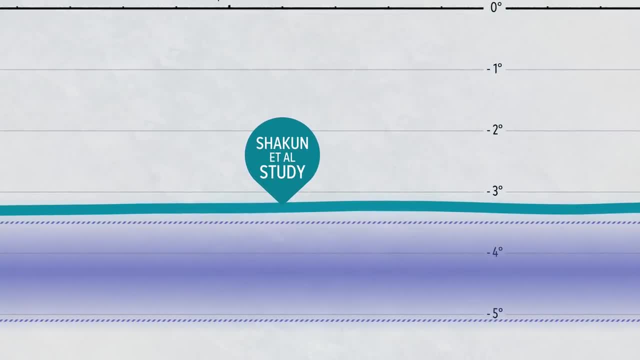 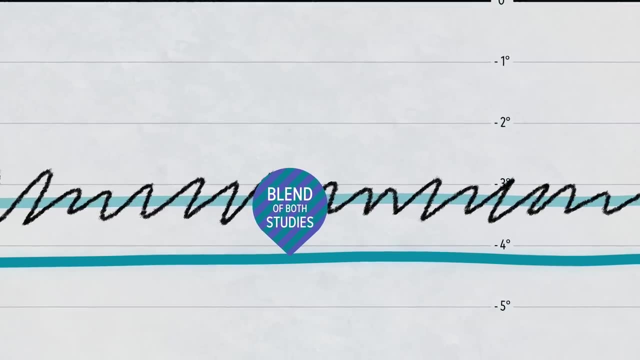 were OK with me using the shape of this timeline as long as it was shifted downwards to agree with the more reliable ice age temperature, And they were not comfortable with me showing numbers pulled straight from the single study. And I wasn't comfortable at first. 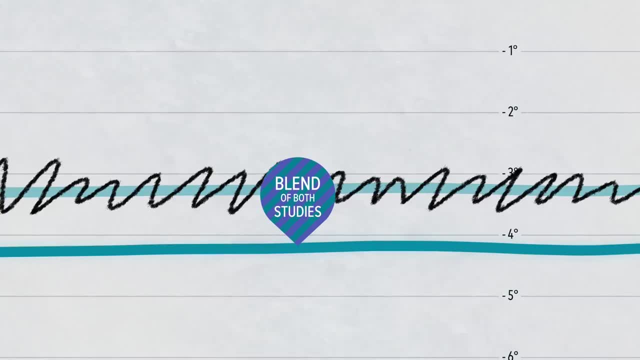 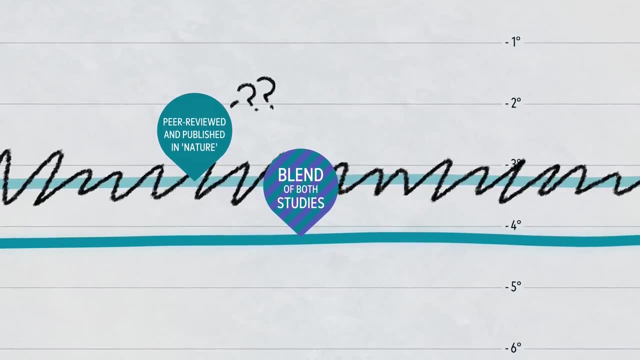 questioning numbers published by credible experts, But that's just it. To improve how health is done, you've got to be careful. The problem is when health and nutrition get reported, journalists need to scrutinize, even filter, what gets publicized, beyond just ensuring. 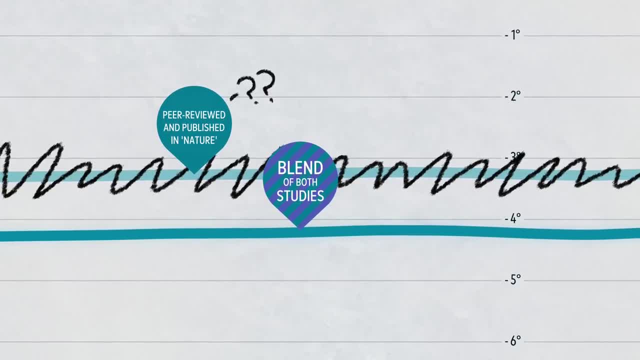 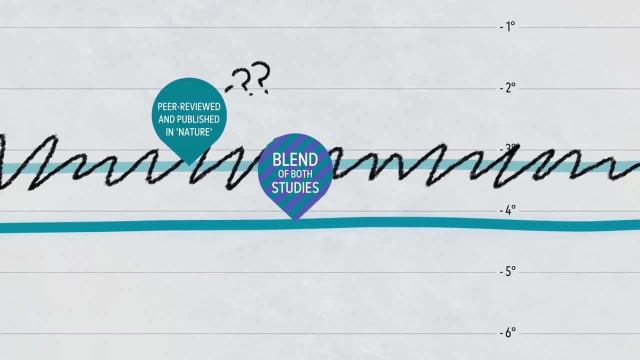 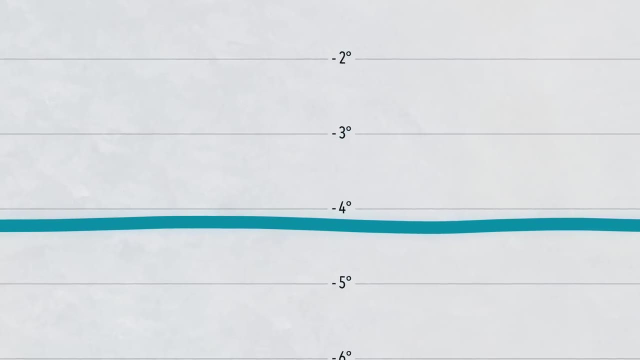 studies are peer reviewed and published in a major journal, Which means people who aren't called scientists kind of have to be scientists. Now, error margins can be misleading for other reasons too. Certainty is often too complicated to be summed up as a simple number or phrase. 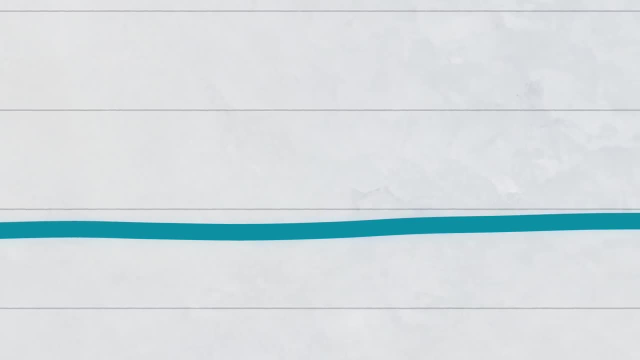 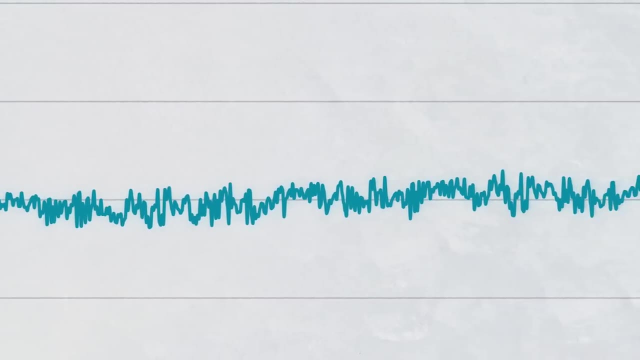 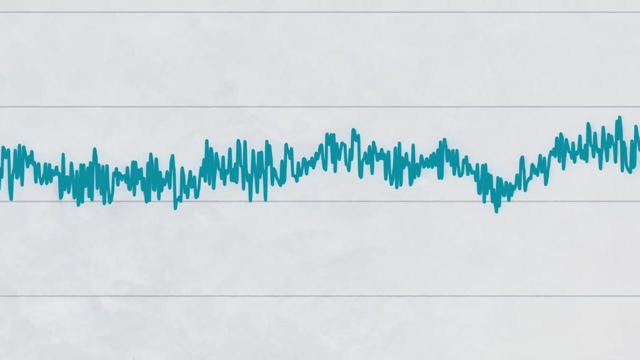 For example, this graph may be too smooth, which, relevant to the climate debate. Short-term variations like this or this could have occurred, but the level of precision in the underlying data kind of blurs the image. Variations. this big, however, are unlikely to have happened. 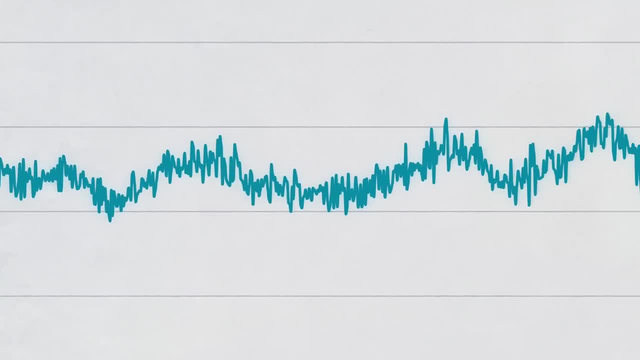 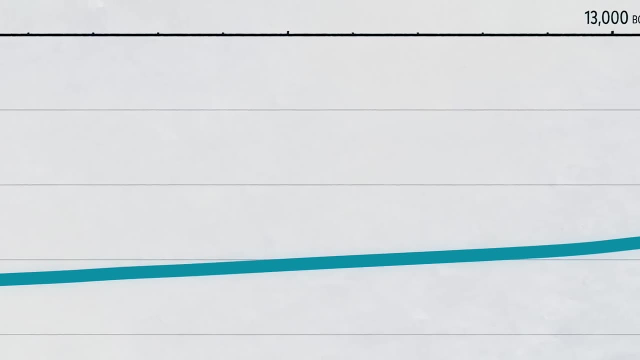 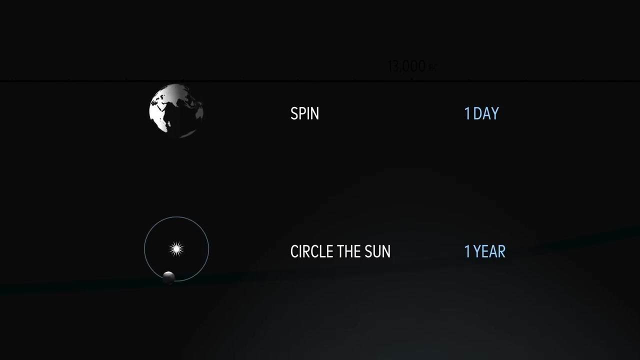 without leaving a mark in the natural record. But a smoothed-over line does show long-term trends and you may have noticed the temperature has been creeping upwards. Do scientists understand why? Well, the Earth's orbit is composed of many different cycles of different duration. We experience the 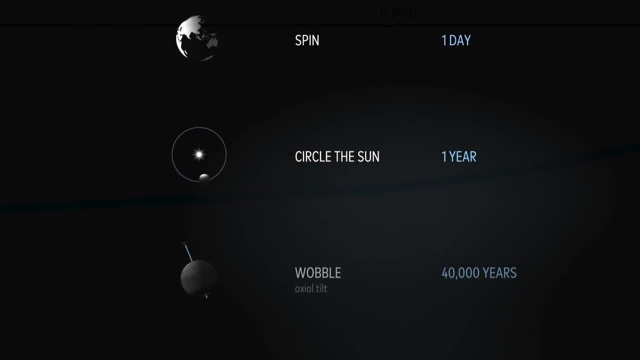 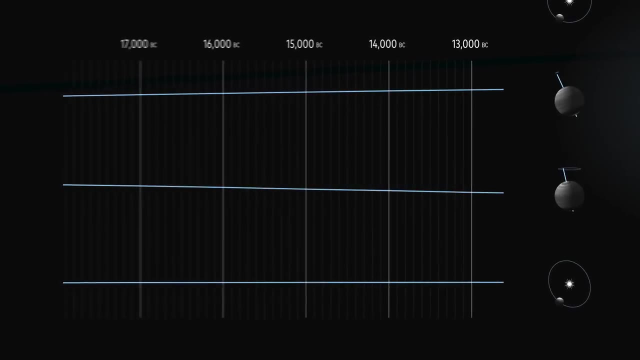 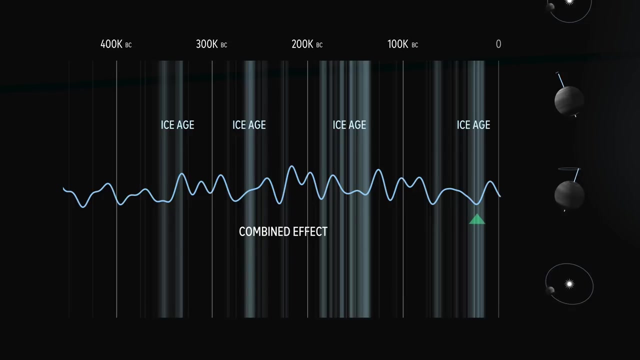 daily and yearly cycles in a dramatic way, But some more subtle repetitions occur over tens of thousands, even hundreds of thousands of years, And the accumulated effects of these long-term cycles tracks, with evidence of ice ages which you can see in some places. 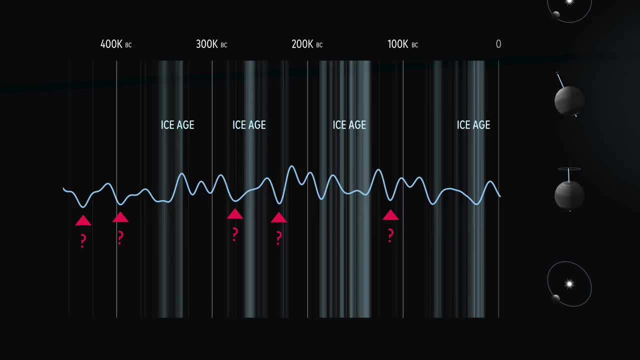 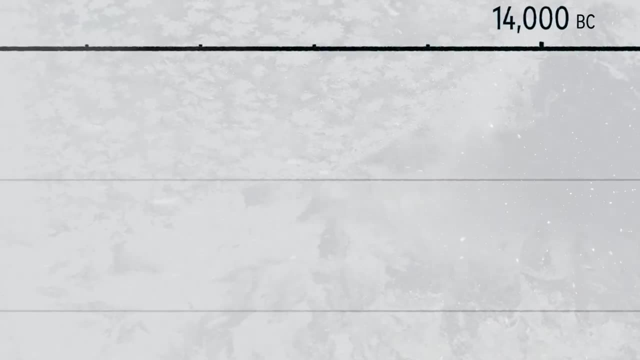 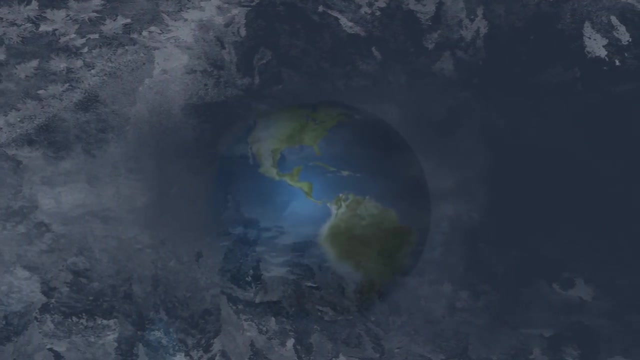 But in other places it doesn't line up that well. Well, that's because scientists explain the relationship is complex. The orbital changes didn't directly cause the temperature to rise, because they didn't cause more sunlight overall to hit the Earth. They did affect the angle of the Sun in a way that allowed more of 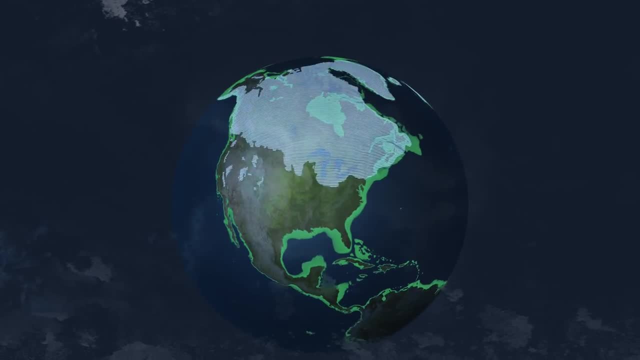 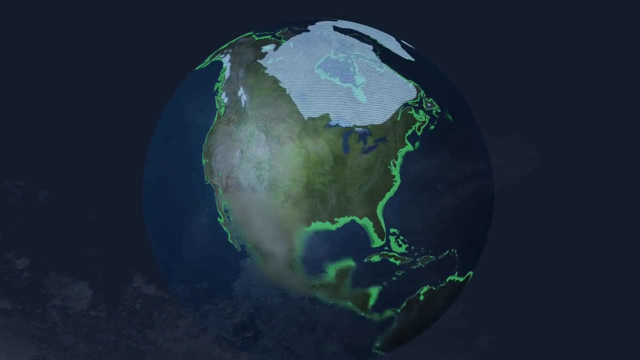 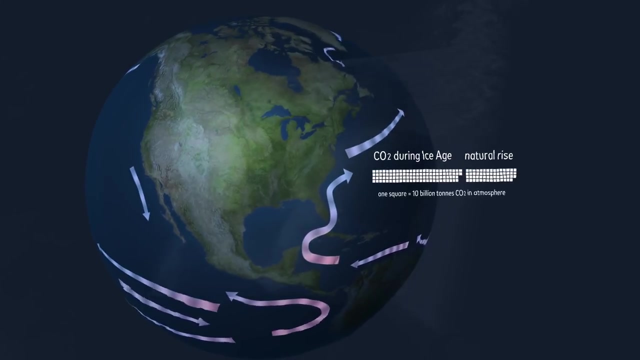 it to reach the poles, which caused the glaciers to retract, which meant the Earth was less reflective, So it absorbed more sun And there were new sea currents And carbon dioxide levels increased, though scientists aren't exactly sure why. And all these? 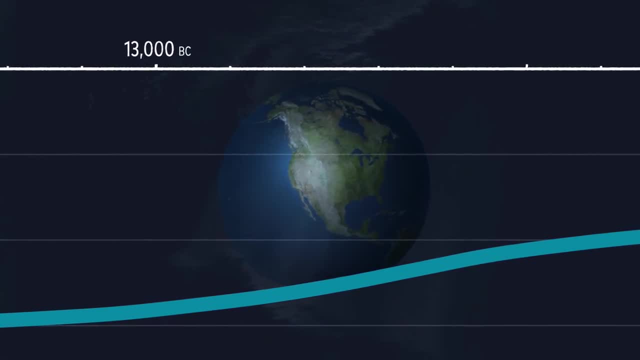 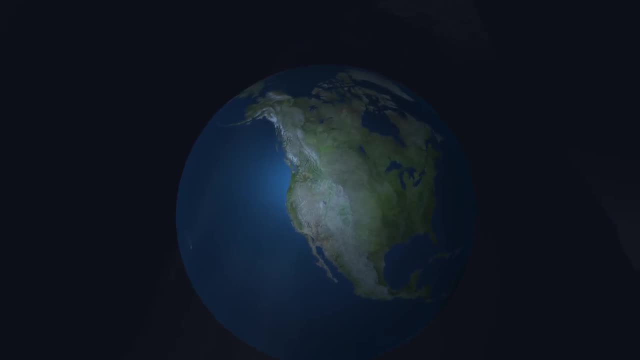 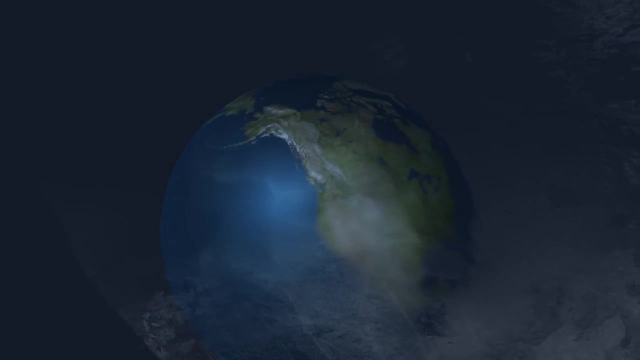 secondary factors cause the average temperature to rise. Scientists say they have a pretty good understanding of this, But even when the world seems to be in clear view, the picture is always at least a little bit out of focus, obscure, distorted. Another reason scientists can't reliably tell us how sure they are is that 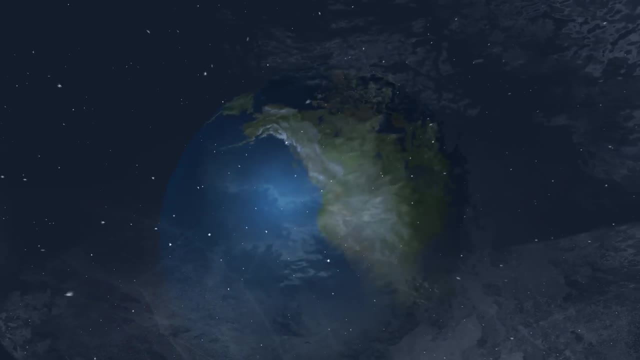 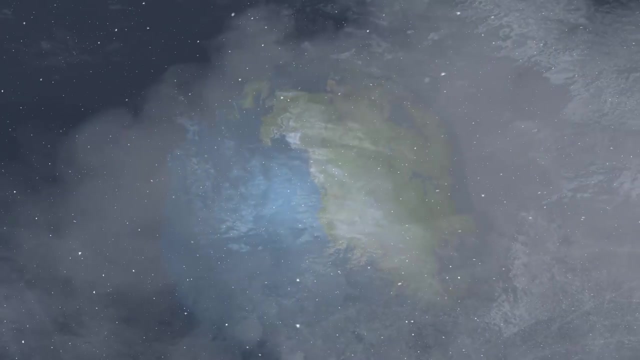 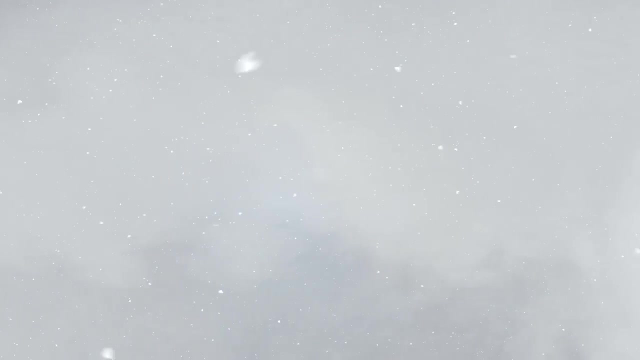 often they don't know how close they are to the truth And they're prone to confirmation bias and often under pressure to publish noteworthy findings. Even the guiding principles of science itself aren't set in stone. Key concepts have been rebuked. 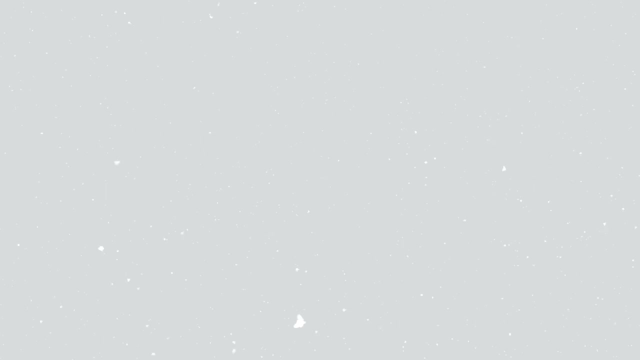 and revised. Until the mid-1900s, scientists believed that discoveries were made by observing their surroundings and making logical conclusions, a process called empiricism. Then they realized that acquiring knowledge was a more imaginative process To cut through the fog. scientists 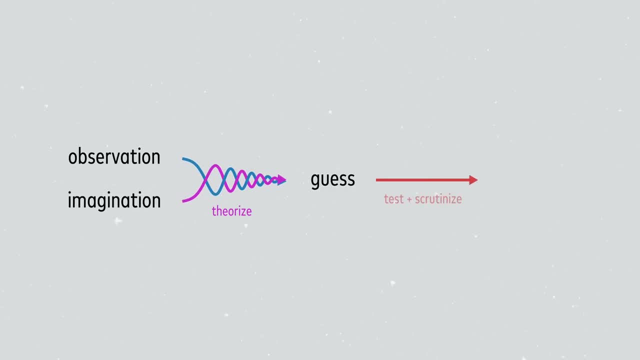 have to make guesses on top of what they know, and then test these guesses, And that's how they did it. So imagination, when paired with scrutiny, is central to the discovery process, And uncertainty, the very thing that clouds our view, also frees us to construct possible. 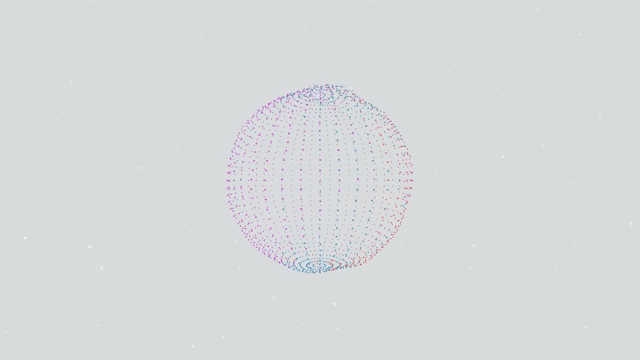 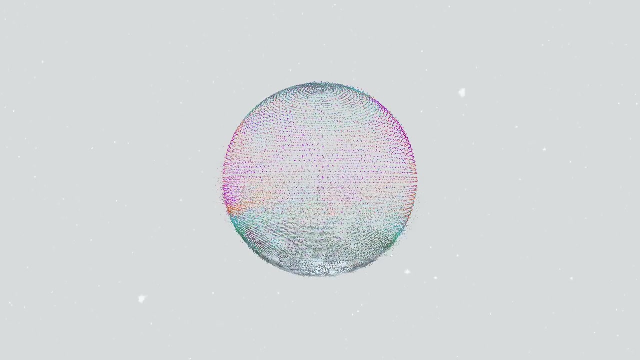 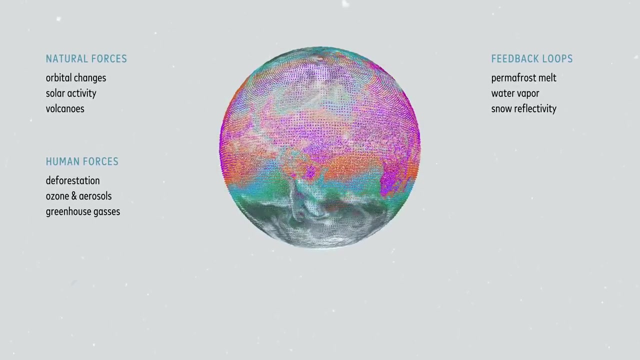 answers. Climatologists have built models that help them predict how different forces affect each other and impact the Earth's temperature. like the way meteorologists use models to forecast the weather, They grow more certain when experiments confirm their theories, when different types of evidence agree and when 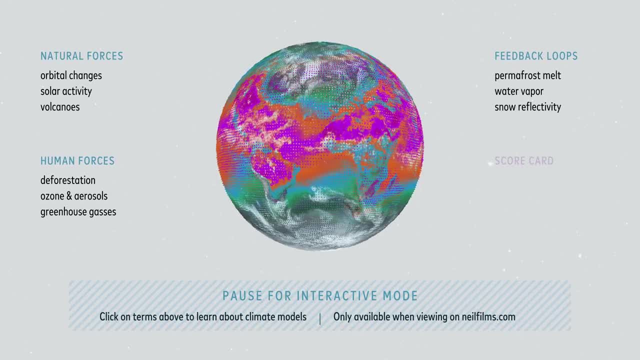 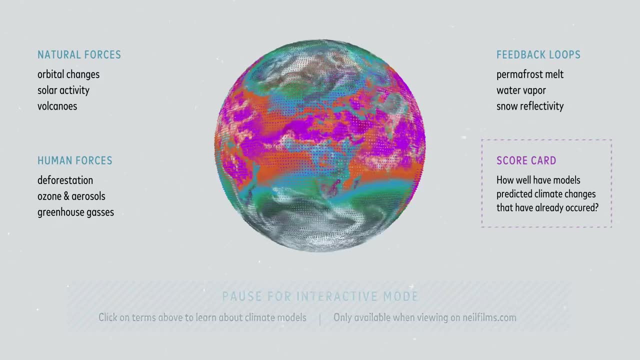 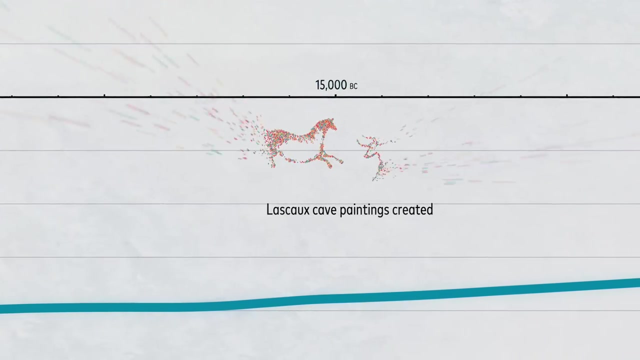 theories survive critical review from others. Plus, these models have been around long enough now that we can look back and see how well they predict the changes that have already occurred. Now let's shift gears and look at what humans were doing since that last ice age: Shrinking. 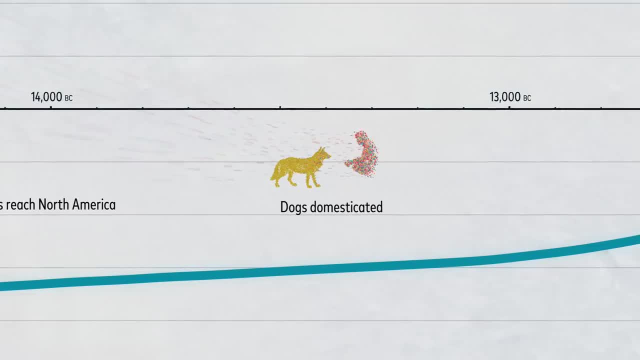 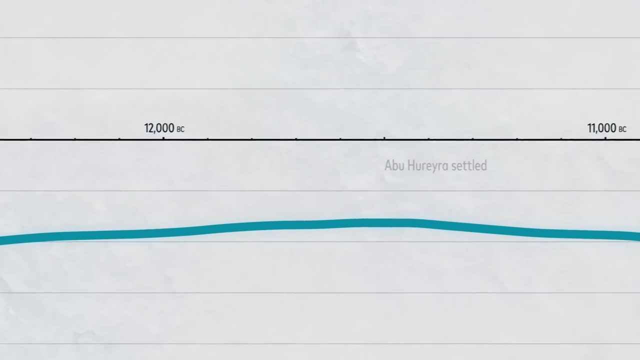 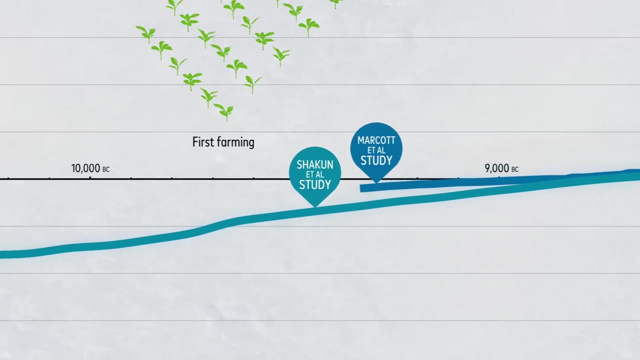 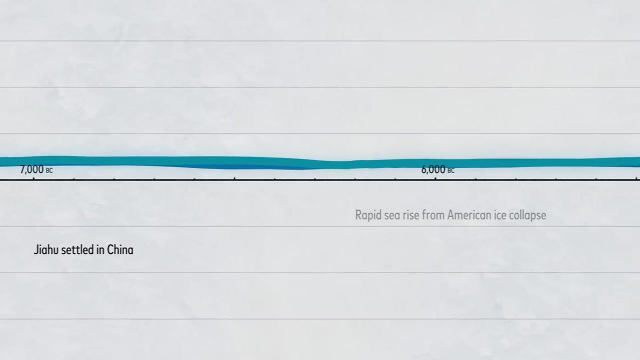 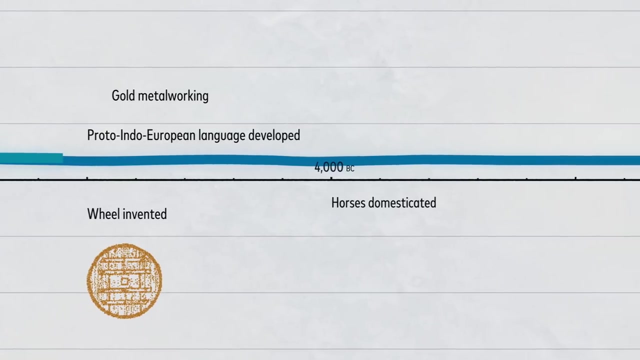 ice sheets allowed humans to cross that land bridge we saw before, You saw earlier, between Asia and North America. Sometimes melting glaciers would collapse, causing massive floods or abrupt sea rise. Farming would ultimately lead to the birth of civilization which spread slowly across the globe. Cities would grow larger, Governments. 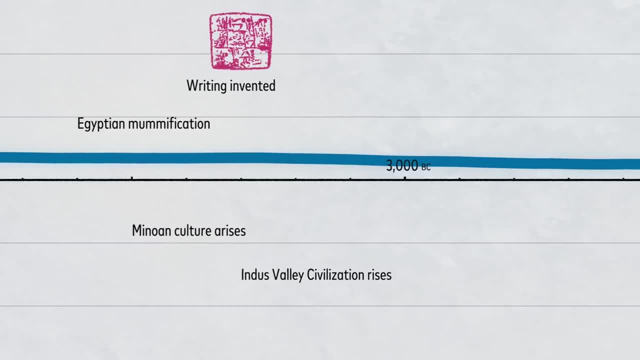 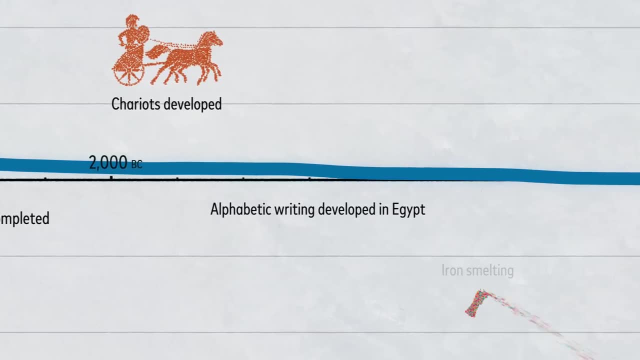 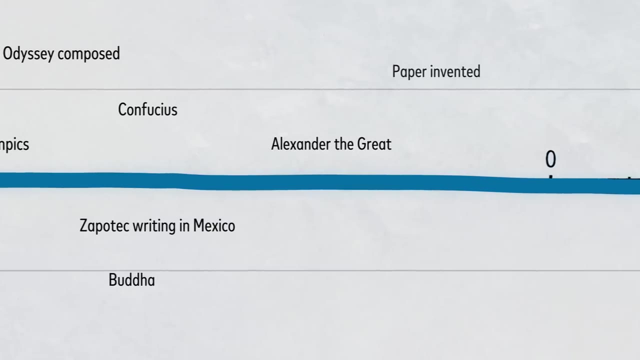 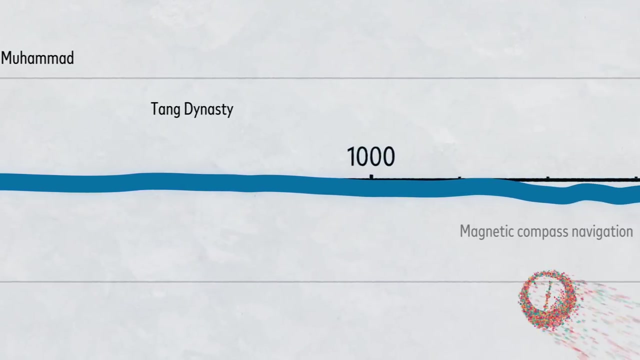 more powerful Empires would rise and fall. So much history happened through these centuries as territories were settled, conquered, reconquered. Big discoveries would change the world, But from a core numbers perspective, the really big changes were about to happen somewhere around here. 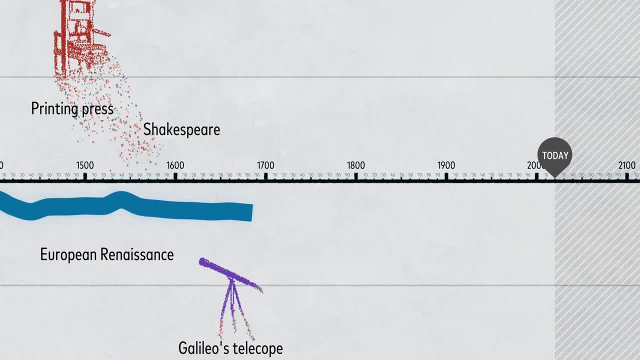 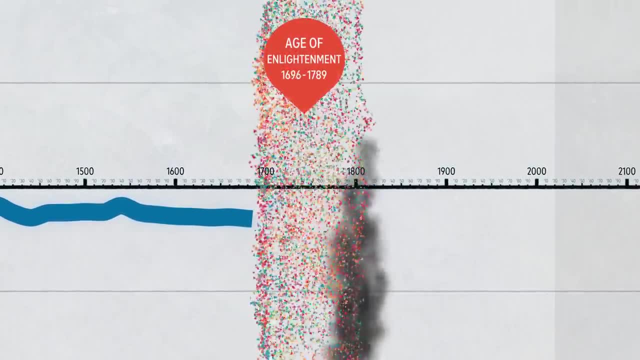 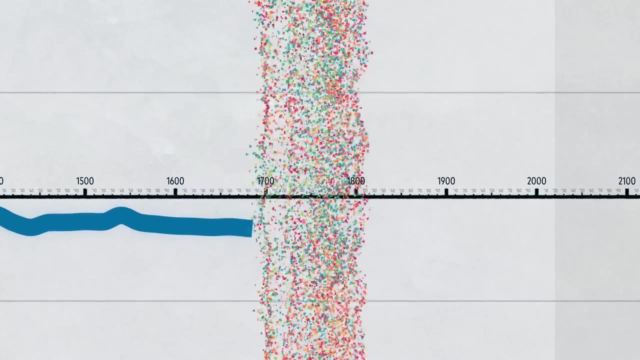 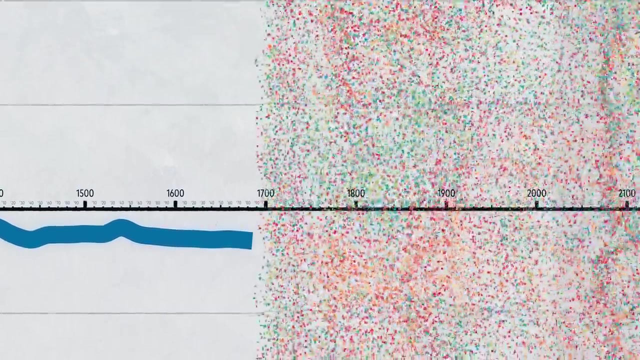 Something dramatic happened: The Age of Enlightenment and the Industrial Revolution. Some say the Enlightenment began around here but never ended. It marked the moment we rebelled against so-called authorities of truth, primarily religious institutions and monarchs. The result was a period of unprecedented discovery. 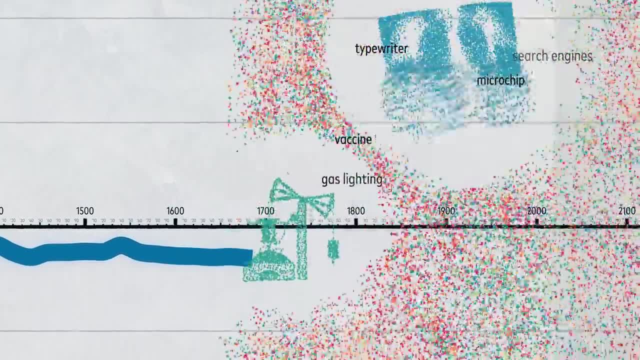 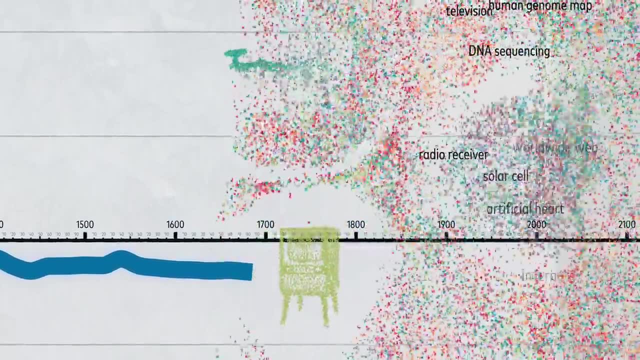 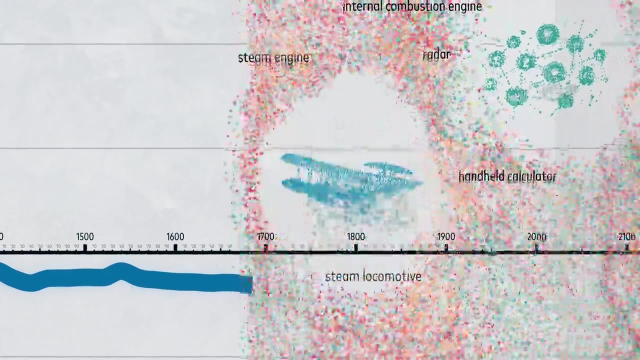 Scientists will say they re different from authorities of truth because they don t want others to take them at their word. They encourage fellow scientists to challenge and test their explanations. As for non-experts, we've discussed how problems can emerge when journalists treat experts. 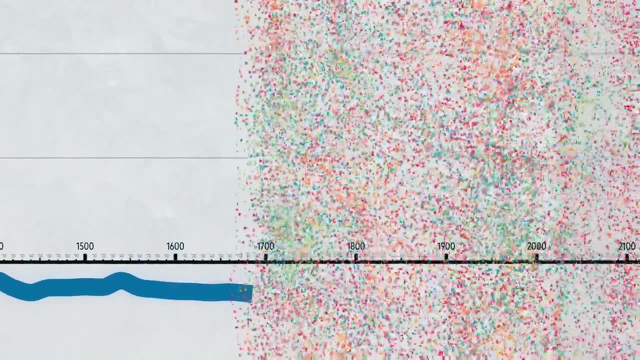 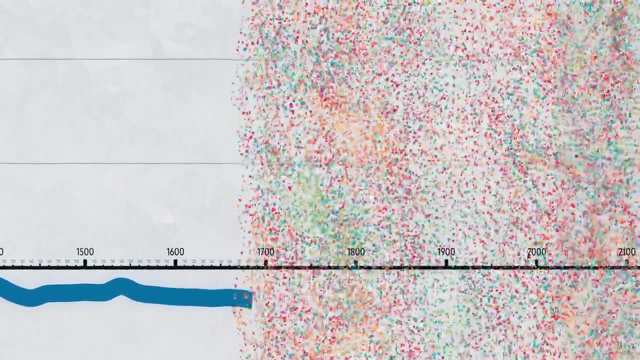 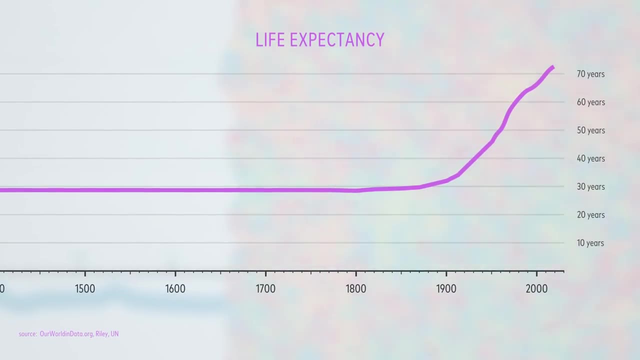 like authorities of truth, And there's a growing concern that, for the public, crusting or distrusting scientists is becoming a matter of history. They are becoming more and more of political identity. Caveats aside, the scientific revolution corresponded with an enormous uptick in human well-being. 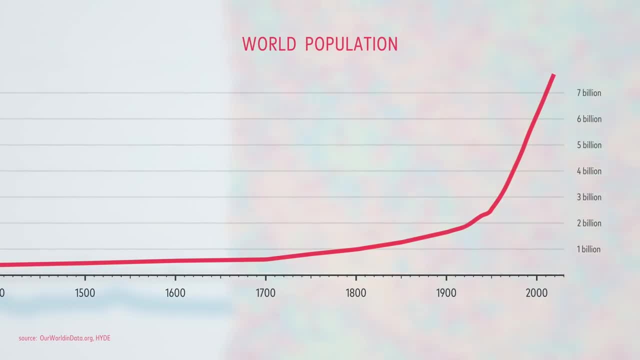 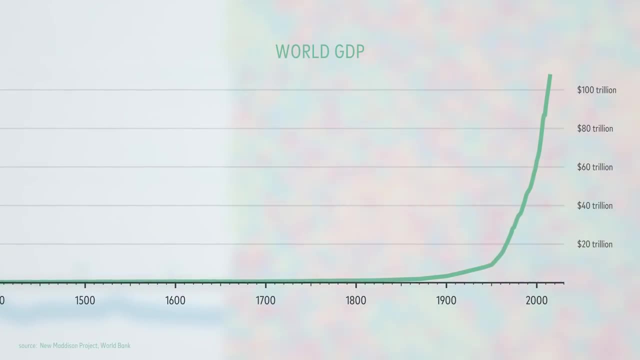 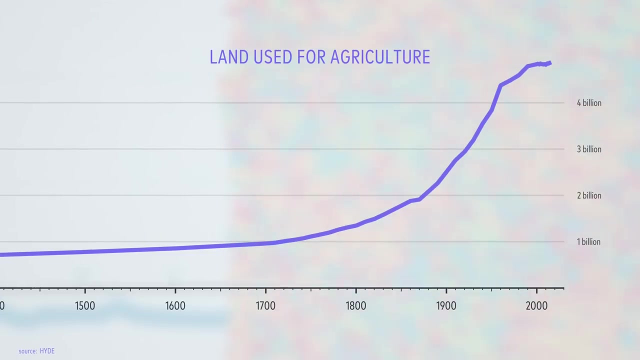 Advances in medicine, agriculture and sanitation allowed us to live longer and healthier lives. Our population exploded. Some might say we thrived, But population growth combined with the Industrial Revolution had environmental consequences. The amount of carbon dioxide in the atmosphere began rising, due primarily to the burning of fossil fuels. 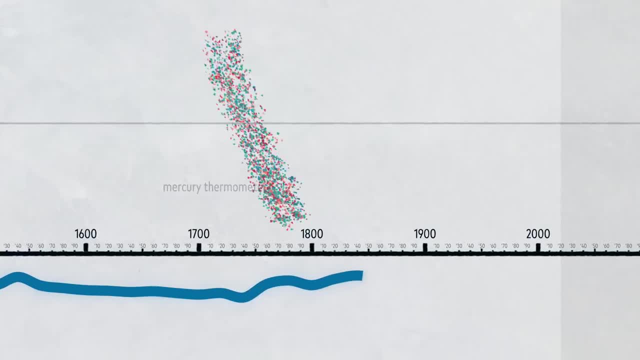 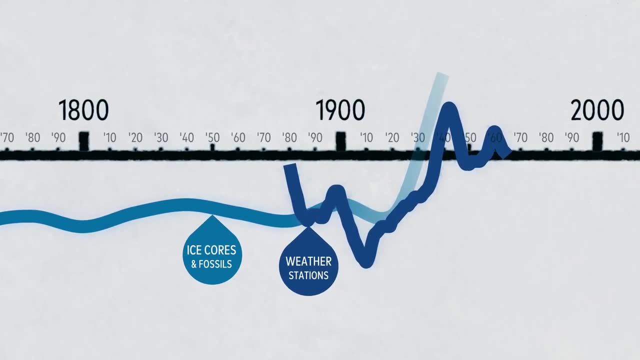 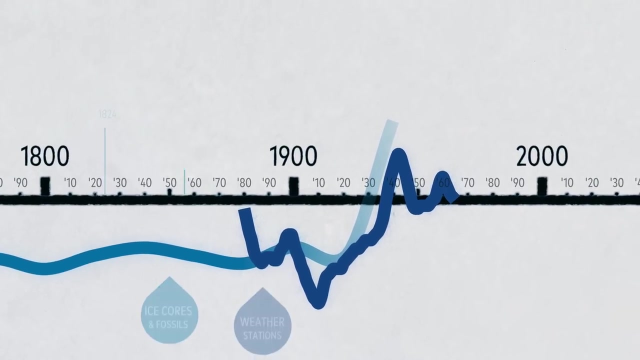 The first reliable thermometer was invented in 1714, which allowed us to collect good temperature data from around the world, And this dark line is NASA's construction of the global average. One could argue that scientists were slow to grow certain of human-caused climate change. 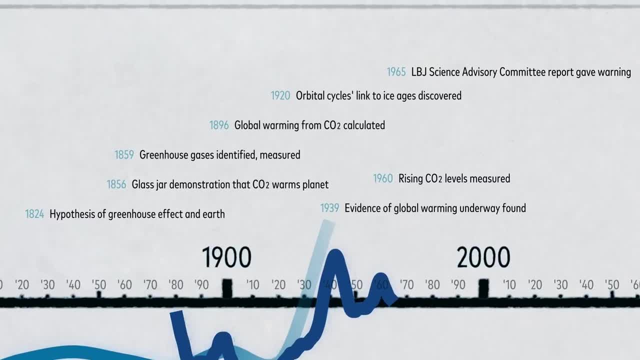 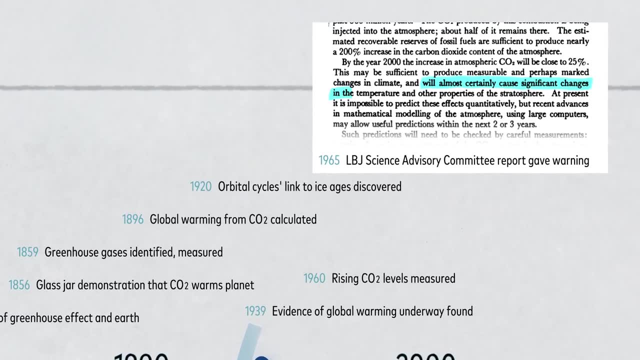 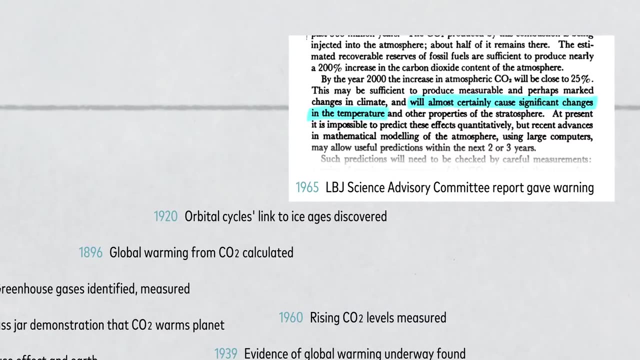 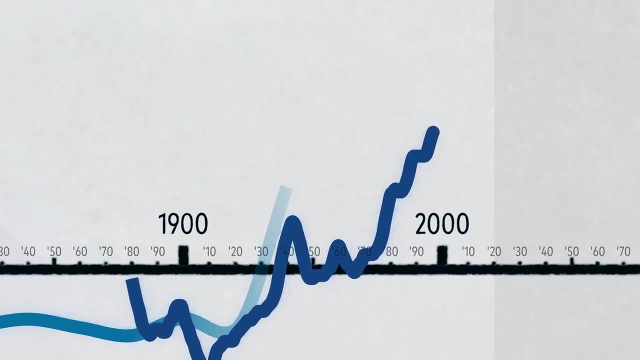 Some studies warned about the problem well over a hundred years ago. In 1965, the US President's Science Advisory Committee issued a major report stating that carbon dioxide quote will almost certainly cause significant changes in the temperature. Since then, the Earth's temperature has been rising. 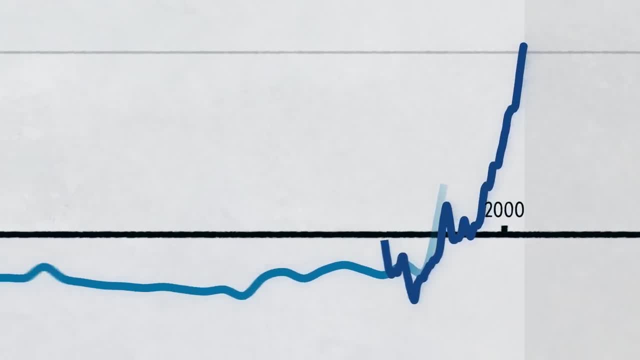 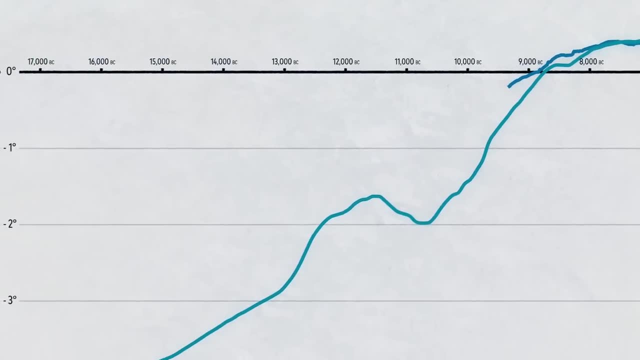 Looking back, the Earth's temperature has been rising. The Earth's temperature has been rising. The Earth's temperature has been rising. Looking back at the 20,000 years we just traveled, the recent warming looks different than past natural changes. Now I've made a point to highlight uncertainty. 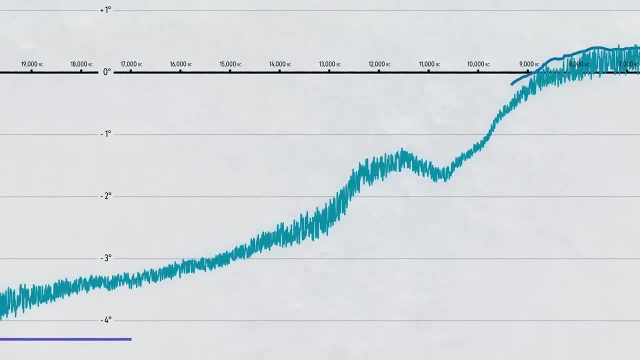 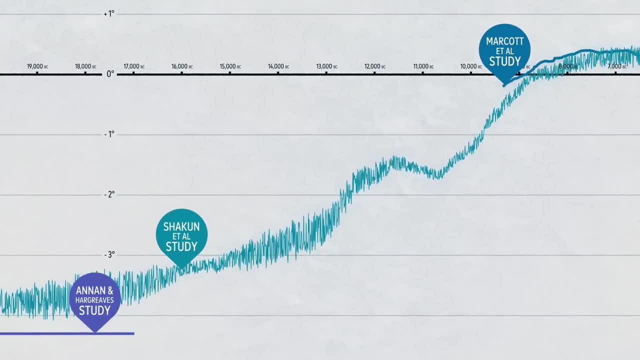 that clouds this chart. Other skeptics have raised other questions, some credible, some not. But you're not a reasonable skeptic unless you're willing to size up your doubts with the larger picture of truth. Uncertainty may not translate into simple numbers. 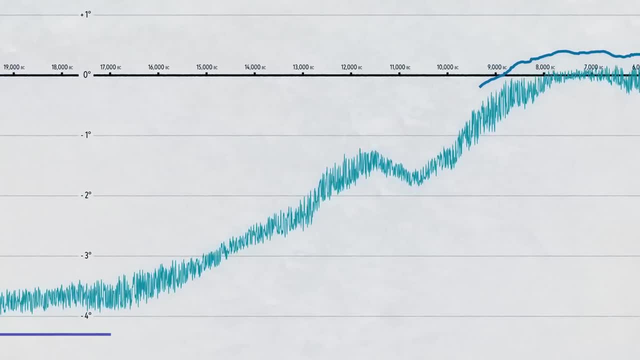 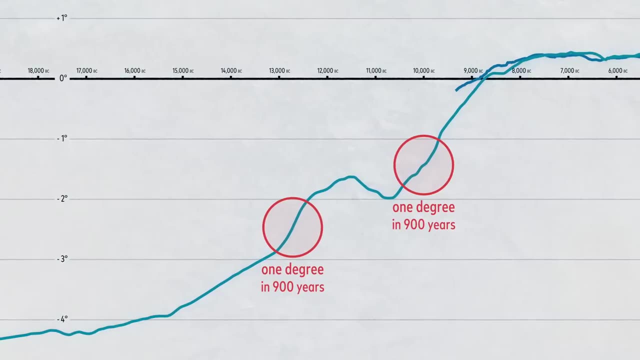 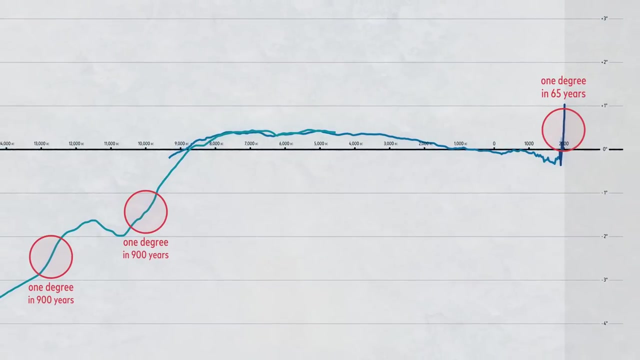 but we can still gauge, as best we can, whether there's enough of it to change the picture. Even compared to moments when we were exiting the ice age the most rapidly, today's rate of warming is of a different magnitude, And it started abruptly when, according to the cycles, 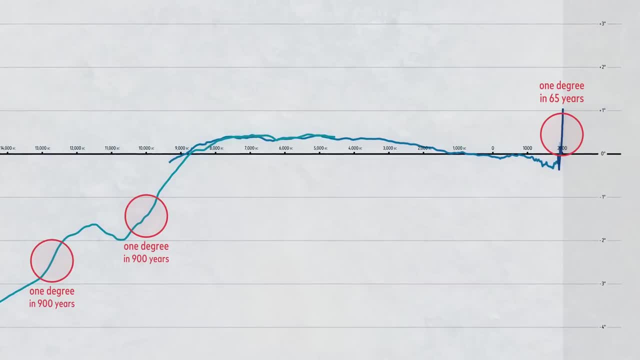 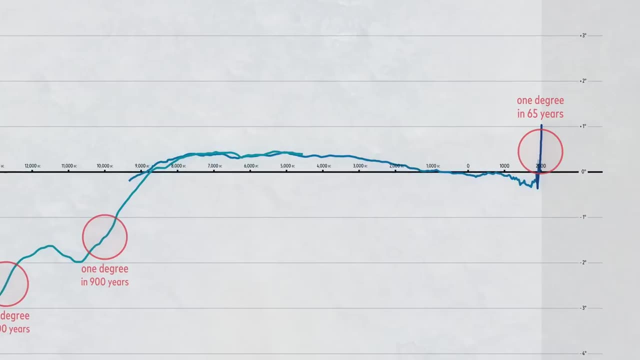 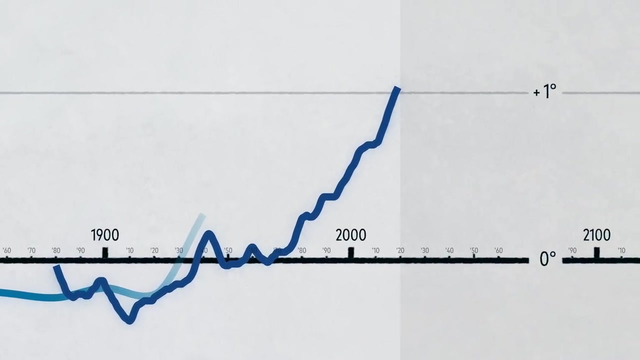 temperatures should be flat or waning, And still, scientists were able to predict it and they explained it with evidence and reason. Now, to estimate future temperatures, climatologists must rely on their models and make a number of assumptions, one being human behavior. 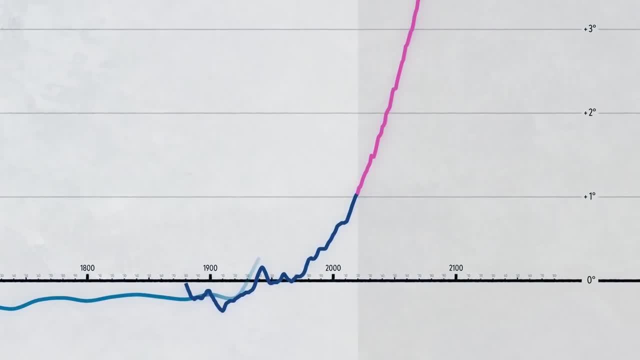 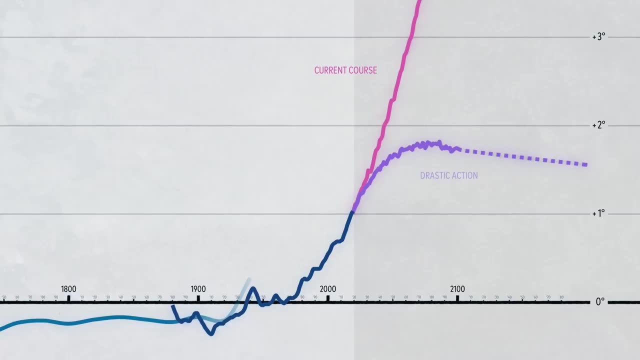 This scenario by the International Panel for Climate Change assumes we make no new efforts to reduce carbon emissions, whereas this one assumes we make drastic cuts enough to keep temperature rise to two degrees above pre-industrial levels And the gap between these scenarios 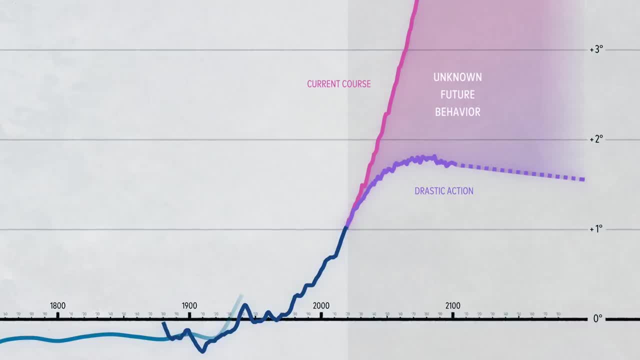 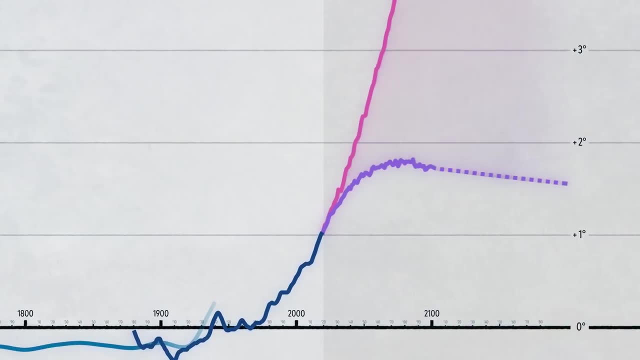 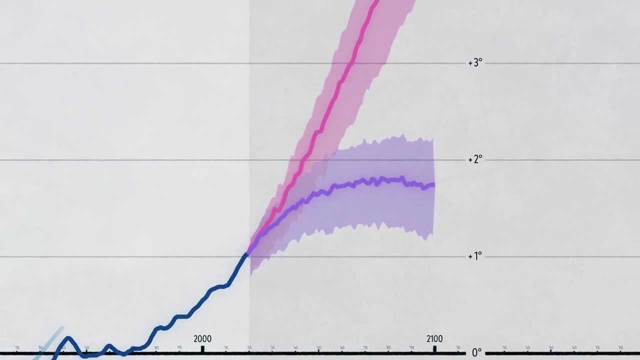 highlights uncertainty stemming from the fact that we don't know what humans are going to do: The realm of soft sciences. But what about uncertainty stemming from the hard science? Well, the IPCC projections do specify a margin of error, which here they get by comparing the temperatures. 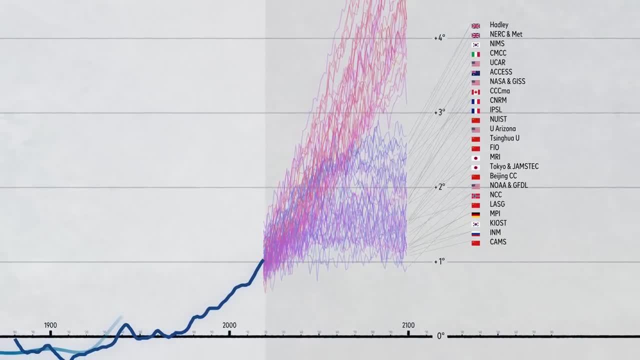 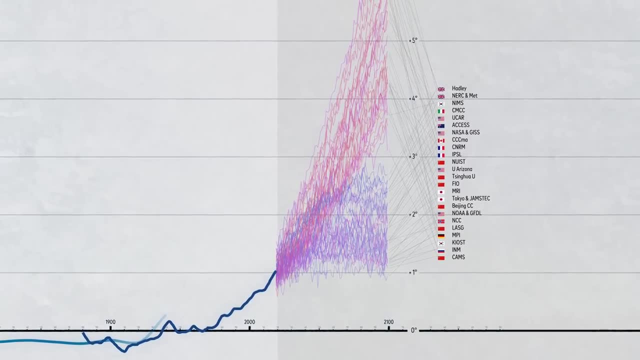 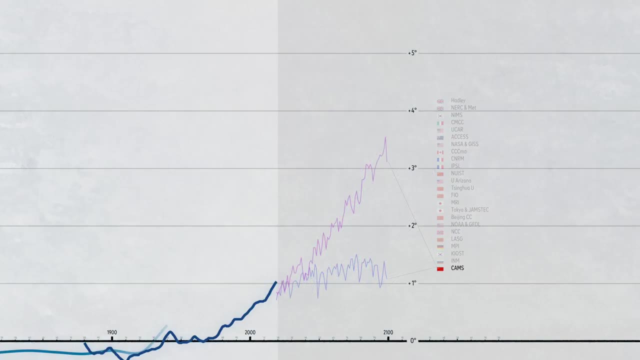 submitted by the teams of scientists behind the IPCC, who've each crunched their own numbers, And if this chart looks messy to you, it is Depending on how the teams designed and configured their models. they got different results, But you can see consistency too. 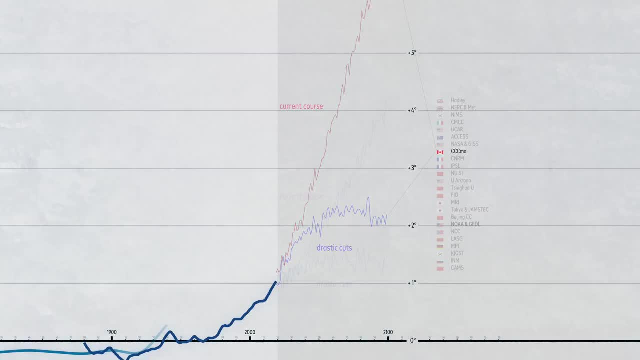 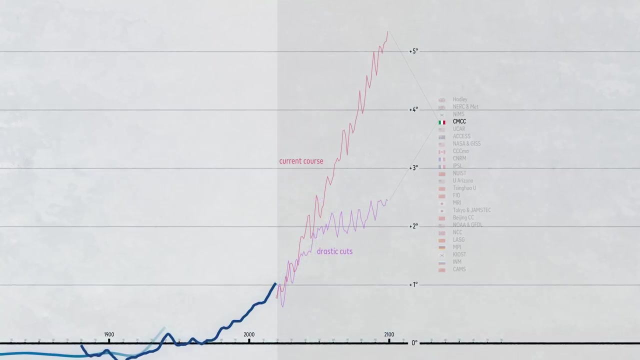 All the teams found that greater carbon emissions will result in significantly higher average temperatures. So even if models can't simulate reality perfectly, they can do it well enough to help us learn and solve problems. And here they're helping us figure out what we need to do. 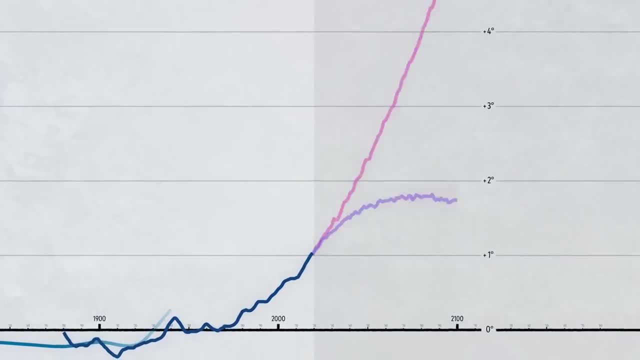 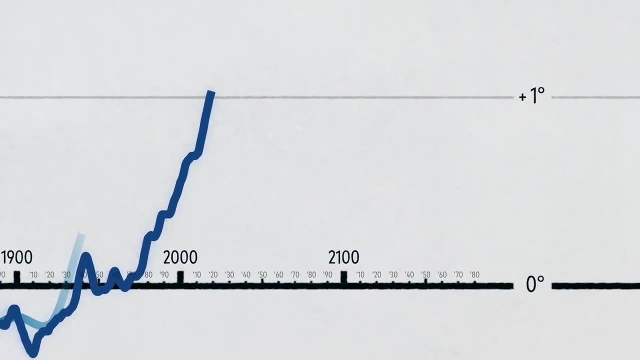 to bring our planet's runaway temperature under control. Now some have argued that because uncertainty is a problem, we can't do anything about it, Because uncertainty exists in the hard science, we should hold back our efforts to change our behavior. In fact, here are examples when prominent figures in the US 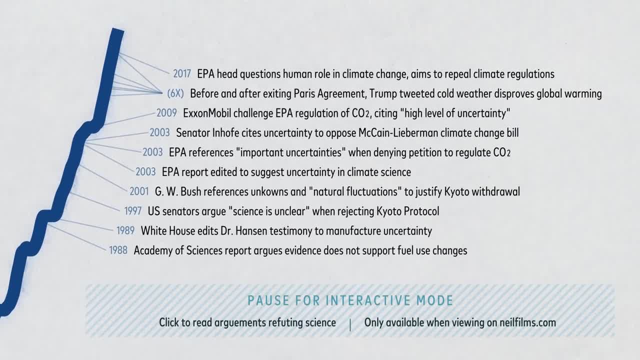 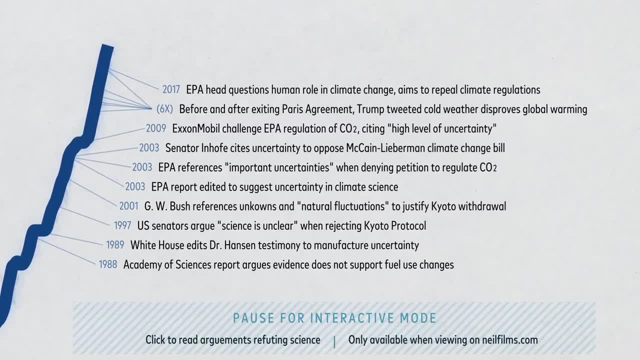 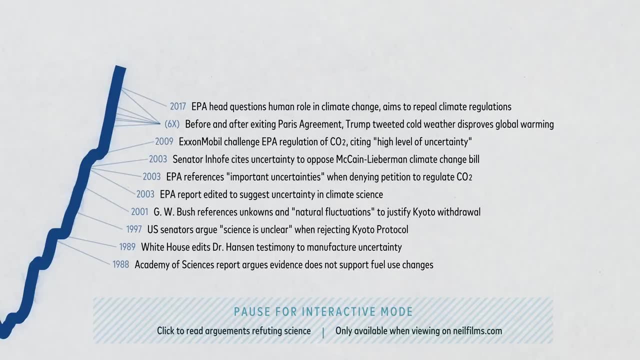 have pointed to uncertainty as a reason to defer policy. Now, if you pause and read about these cases, you might find that many look more like political maneuvers than honest arguments about the science. Still, uncertainty is a prevailing theme of the climate debate. 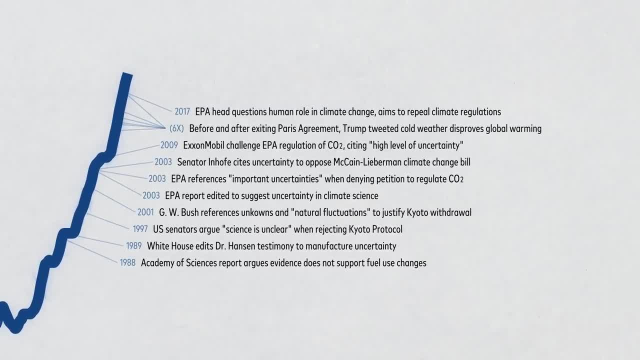 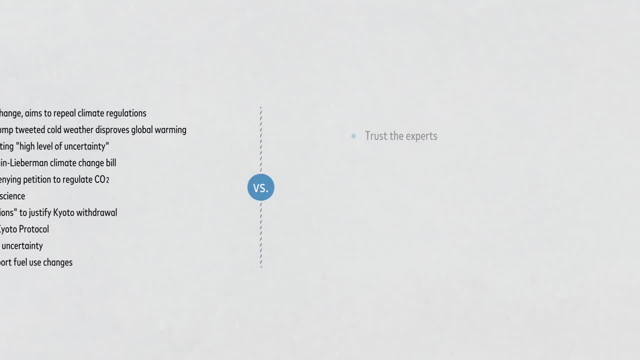 And refuting these arguments with reason takes some work, especially because uncertainty is confusing even for the experts. A simpler rebuttal is to say: we just need to trust the scientists. We can point out that they know the subject matter, that there's a consensus within the field. 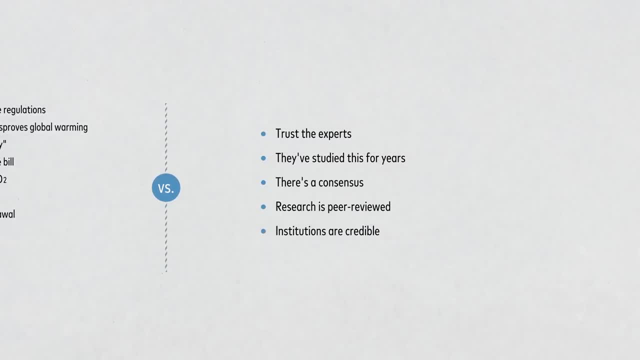 and a peer review process and that credible institutions back their claims. Now notice: these arguments are all about endorsing the experts, not about the mayor, the president or the government. They're all based on the merits of what the experts are saying. 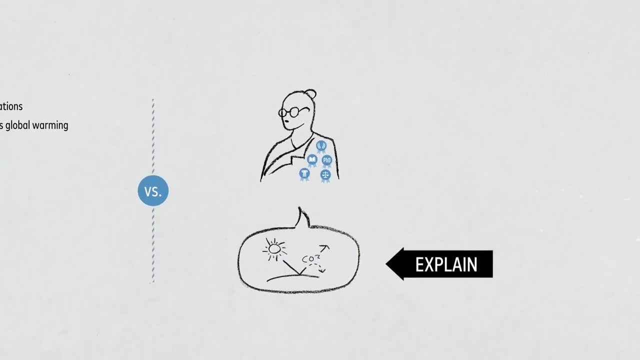 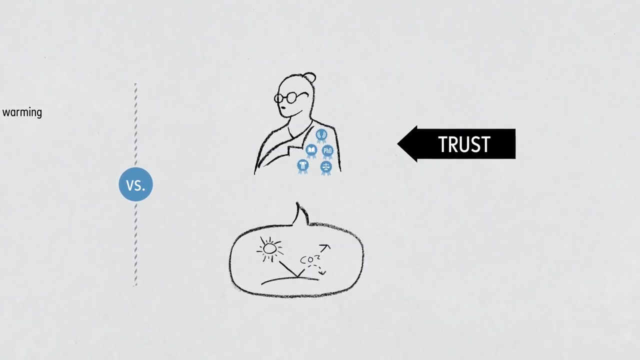 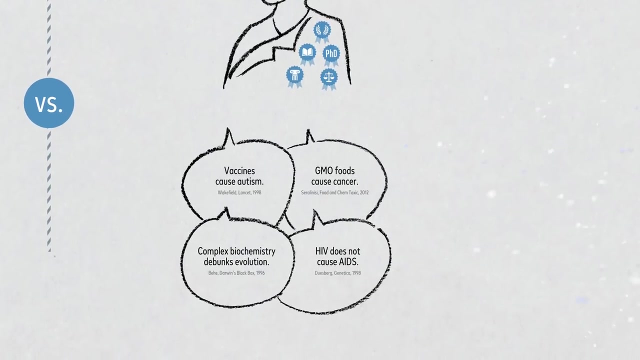 or the science. There are lots of good reasons to trust experts. I mean we have to. Our society functions thanks to specialized occupations, But when somebody questions whether a finding is true, saying trust the scientists is a problematic answer Because we know individual scientists are fallible. 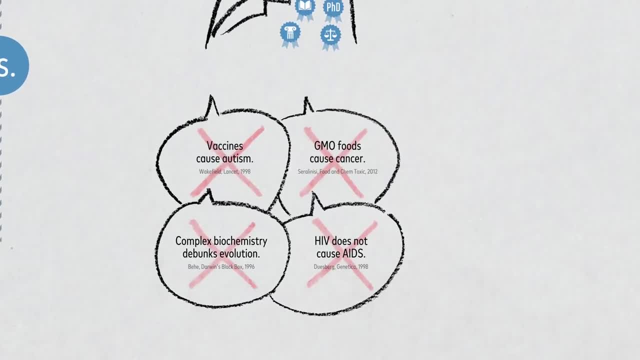 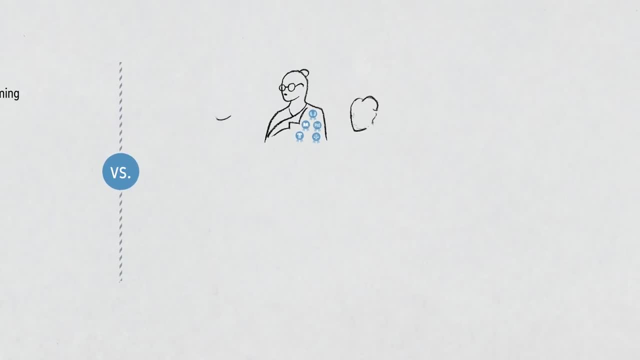 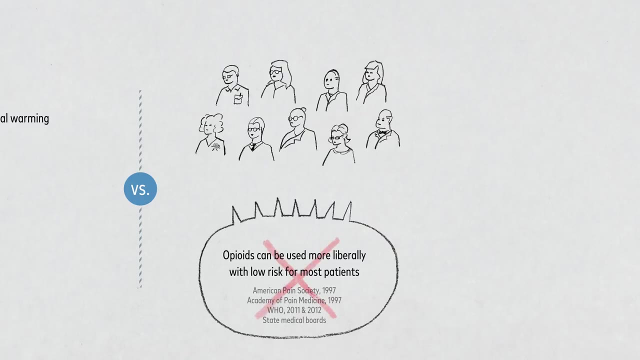 and that individual studies have made false claims And, more importantly, that systemic problems have led influential groups of scientists to make mistakes. And we know that the scientific revolution was built on the idea that we don't take people at their word because we reject authorities of truth. 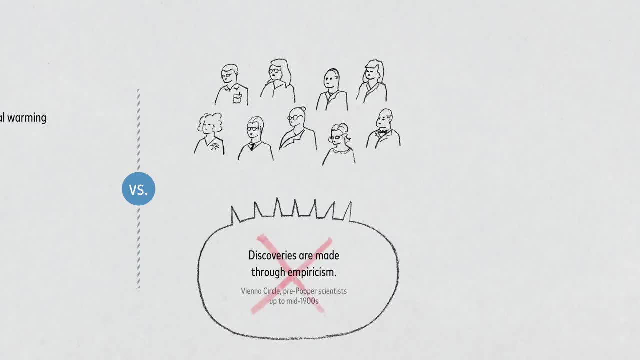 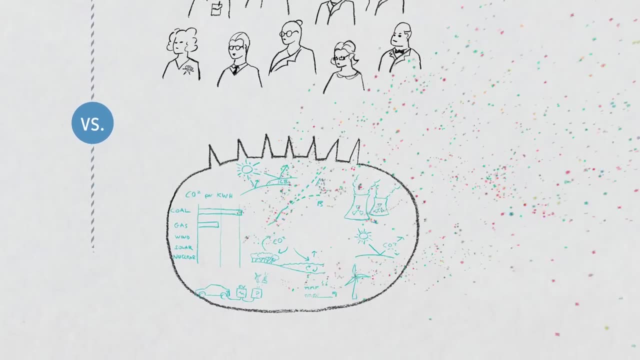 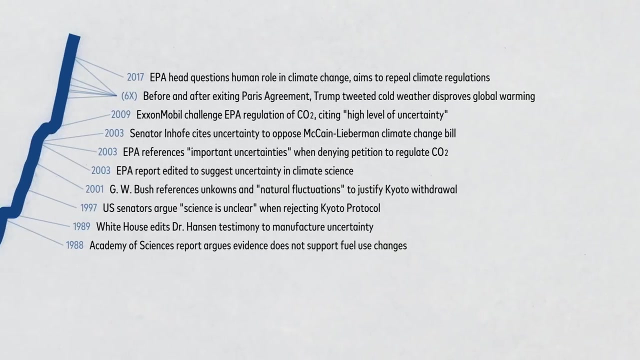 Which is why it's so important for non-experts to, on occasion, wade into the science, Not with the aim of understanding an issue completely- That's impossible- But enough to understand why say these claims are unreasonable. And a beautiful thing happens when we point out: 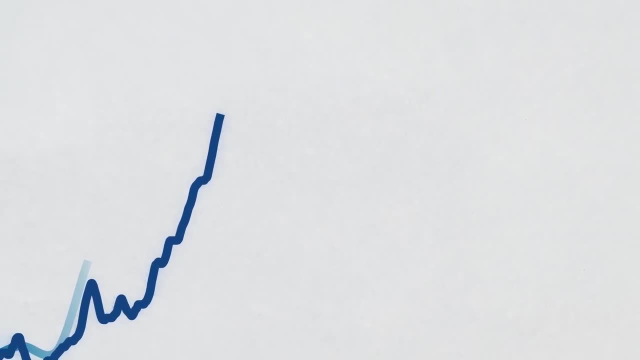 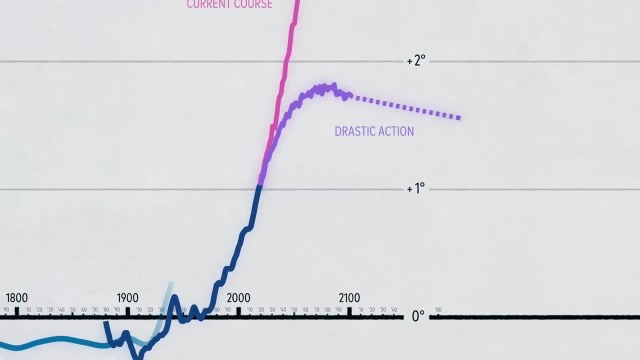 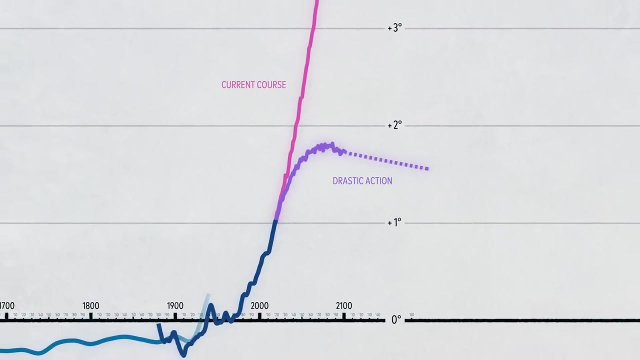 that scientists and their ideas are fallible. We're reminded that we can get better at science And better at explaining science And better at determining, as a society, when scientific claims can be believed with confidence- Enough confidence to take action, as is clearly the case with the climate. 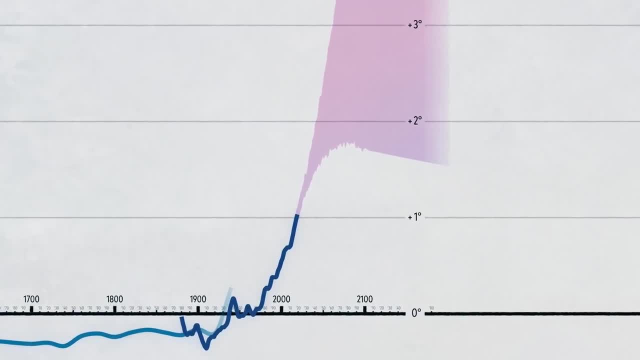 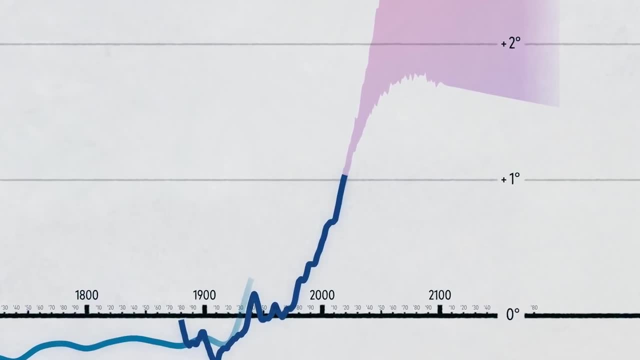 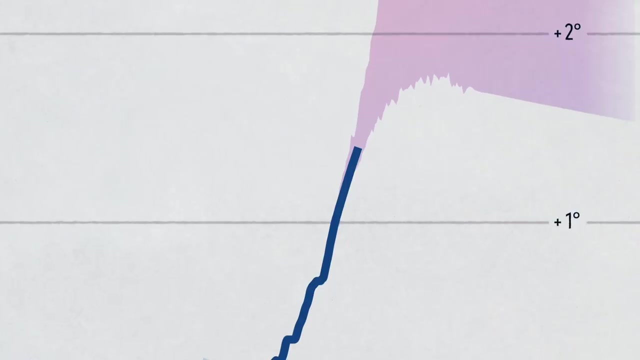 Mind you, people with and without PhDs are prone to over-reliance Or over-confidence when predicting human behavior, And this false sense of knowing people can take many forms. I personally struggle with climate defeatism, A feeling that this line has already been drawn. 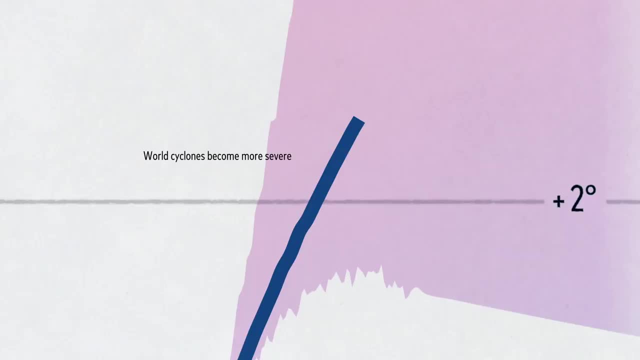 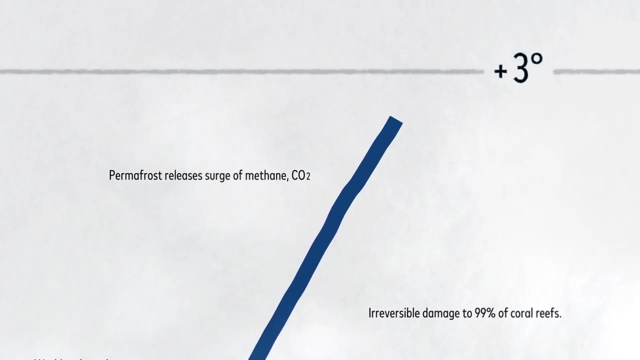 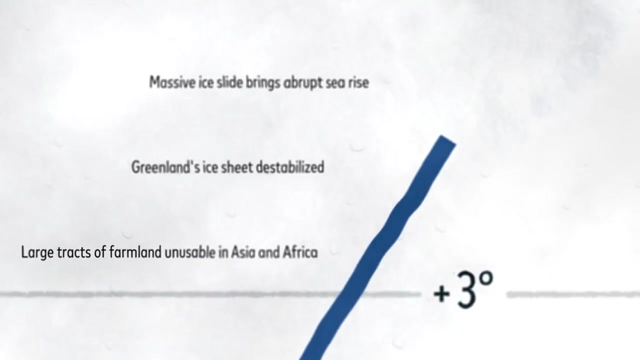 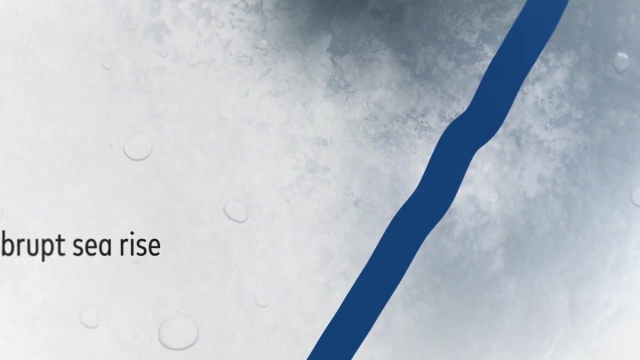 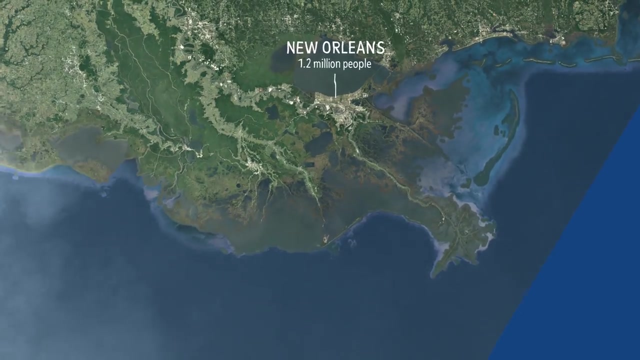 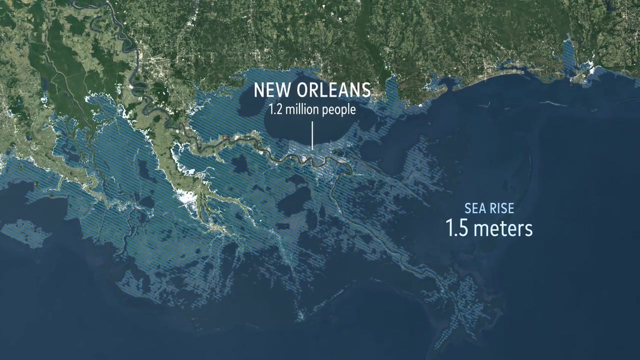 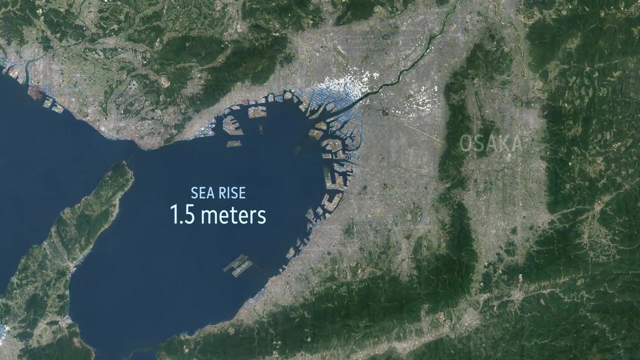 Since, realistically, humans won't change quickly enough to dramatically bend its shape. And without a drastic bend, efforts to fight climate change will only delay the inevitable. And without a drastic bend, efforts to fight climate change will only delay the inevitable. And without a drastic bend, efforts to fight climate change will only delay the inevitable. 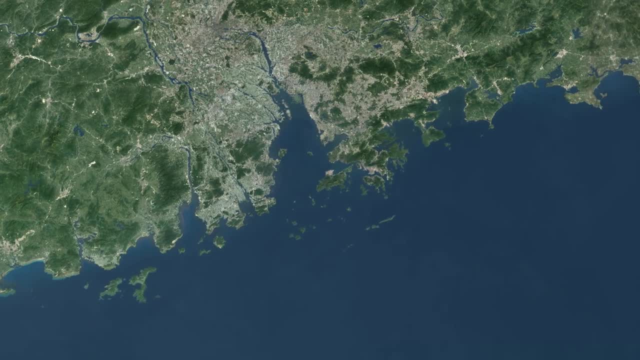 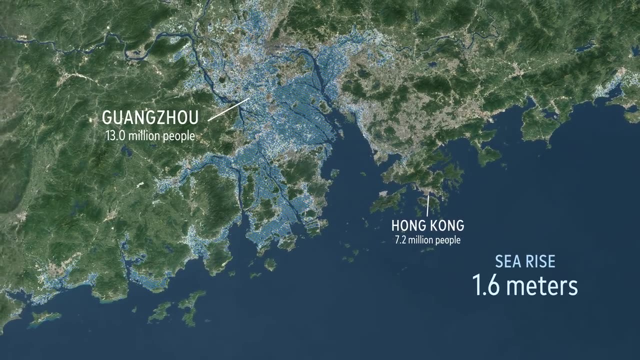 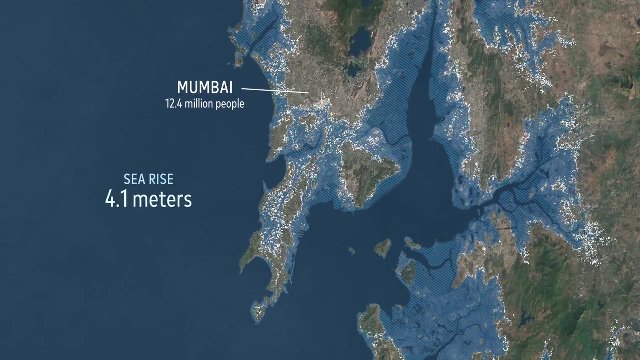 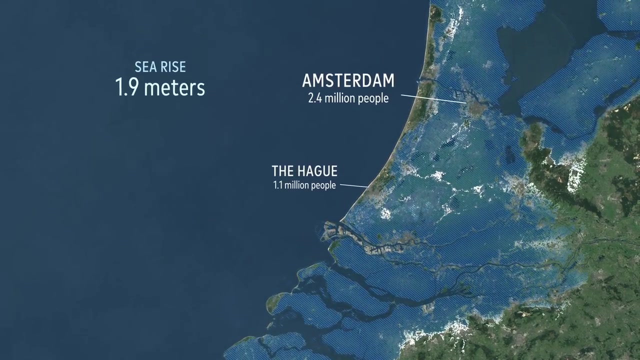 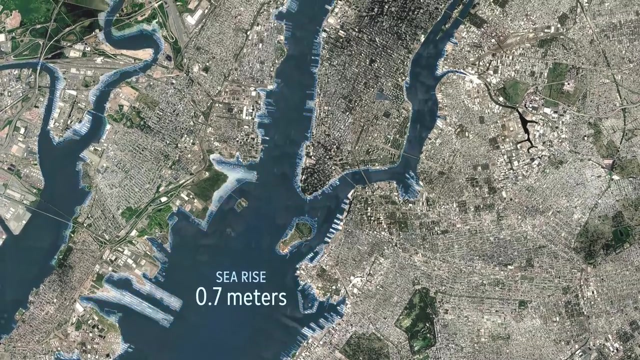 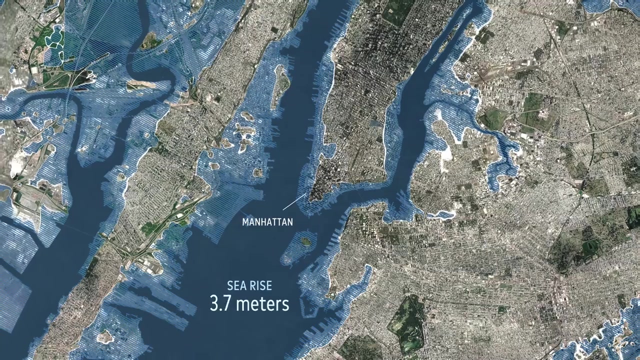 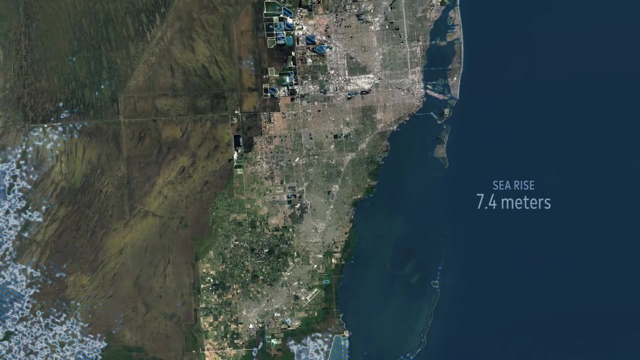 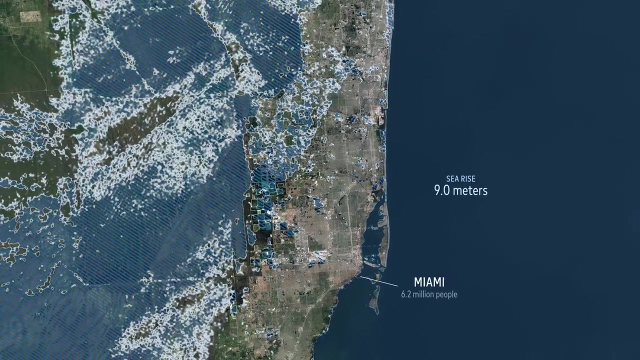 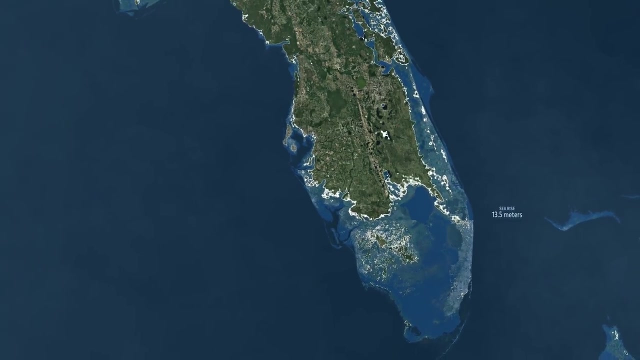 Defeatists might take comfort in inevitability the way denialists take comfort in uncertainty. It takes the pressure off. We defeatists may call ourselves realists, but really we're just overly certain, Perhaps unimaginative Scientists. a century ago, the empiricists were wrong about how discoveries were made. 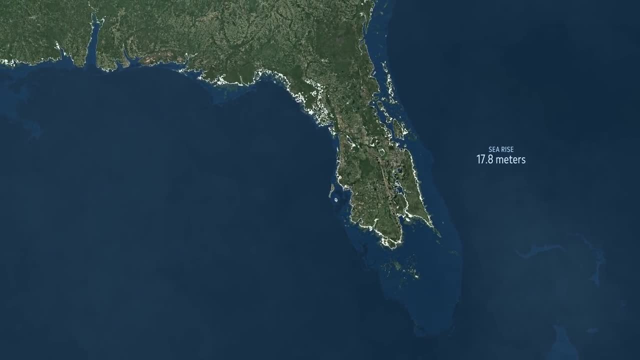 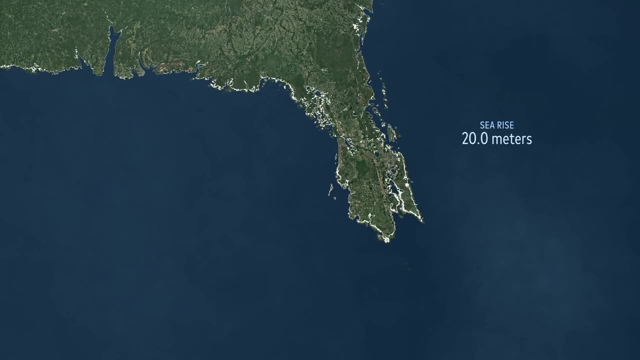 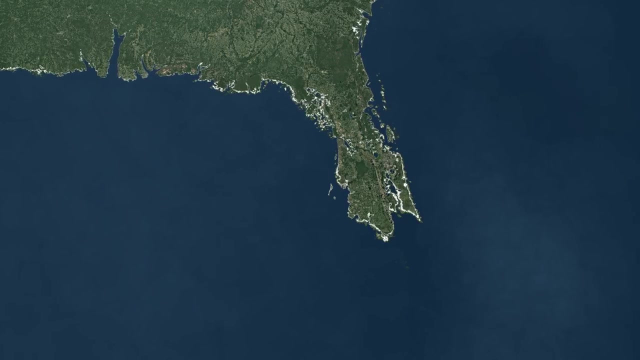 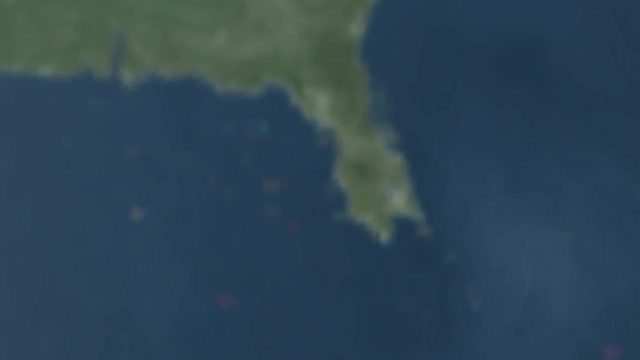 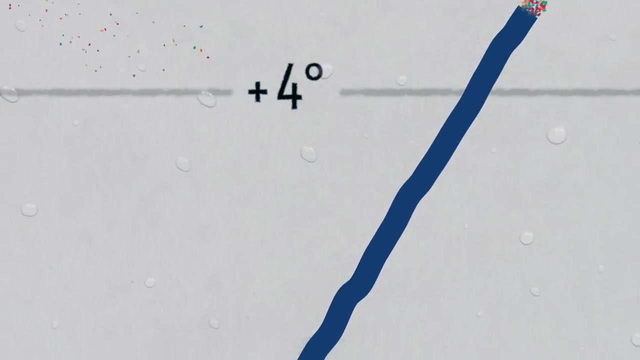 Because they didn't appreciate how important imagination is, How it allows us to reach out beyond what we can see and compose answers Even about things that we don't know, Even about things that were true all along: Laws of nature. So surely imagination, grounded in hard science, knowledge, can be of use when forecasting a future of our own making. 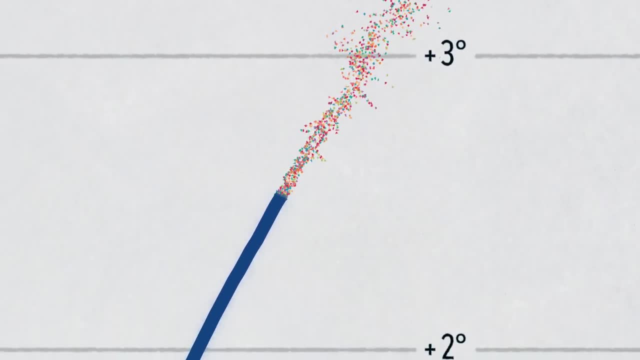 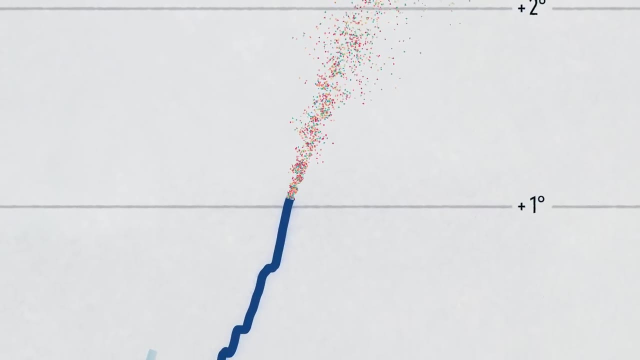 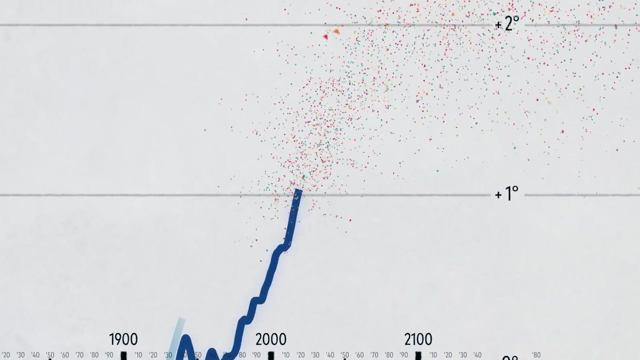 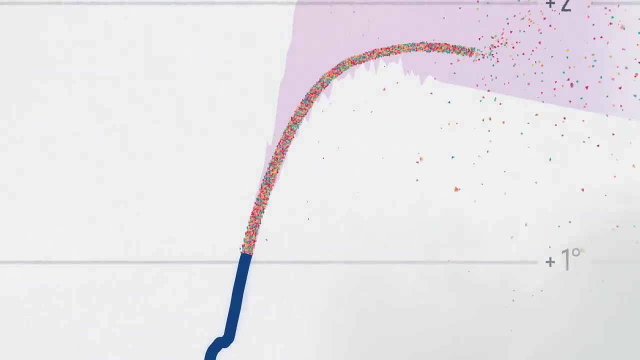 But to devise and then rally behind a good plan, we first have to believe- And I mean really believe- That our future is uncertain, Because only then might we be so bold as to shape it. I'm going to follow up this video by looking at ideas for tackling climate change.